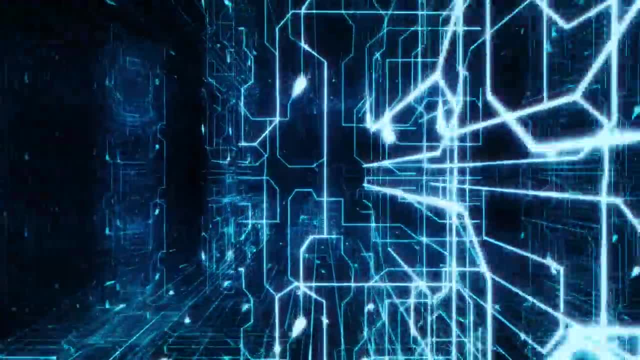 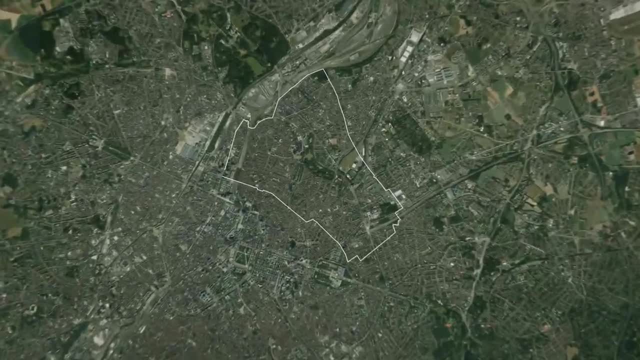 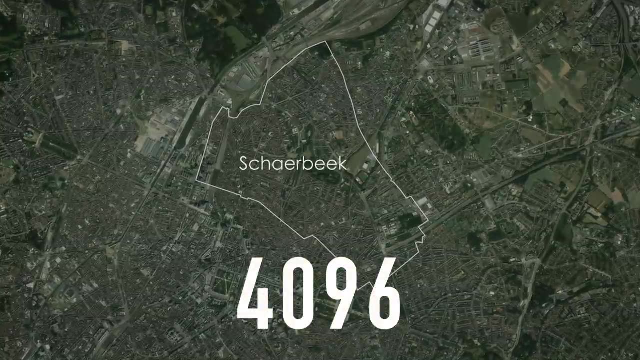 the error. Everything about the hardware seemed to be in perfect working order, And this left only one possible explanation, and it is seriously weird. The clue comes from the excess number of votes. Vindavogel received 4,096.. Computers work using binary strings of zeros, and 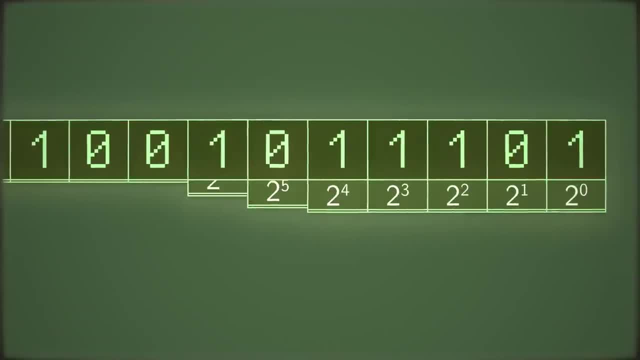 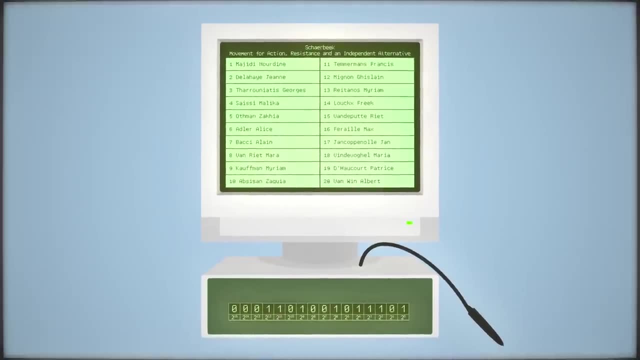 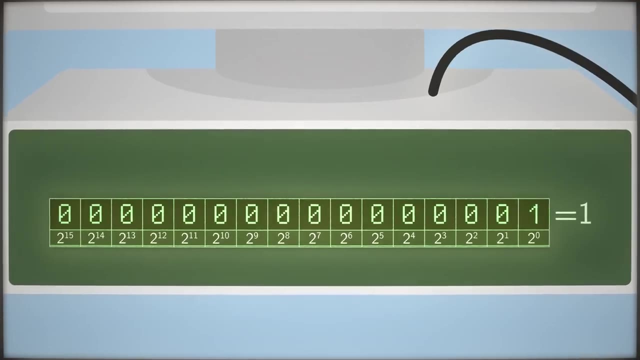 ones, each corresponding to a power of two. So somewhere inside the computer tabulating all the votes was a string of bits representing the number of votes Maria received. It started the day all over again. As each vote for her came in, it would increment by one. Physically, this is done by: 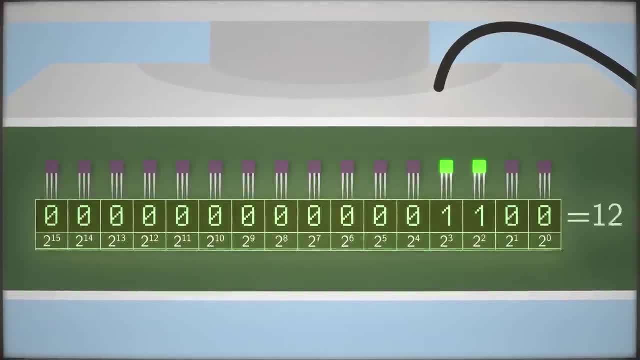 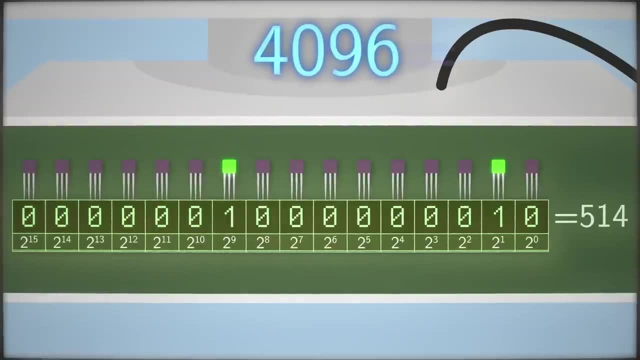 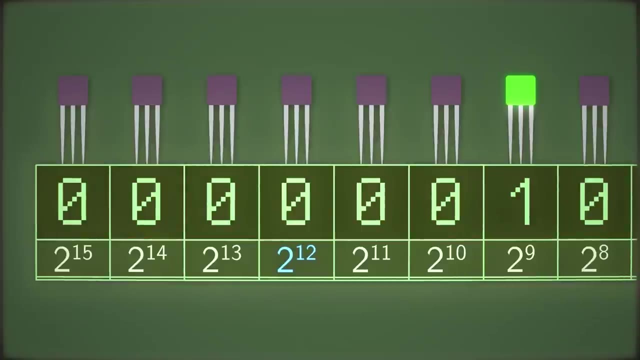 turning on a transistor for one and turning it off for zero. What's remarkable about the number 4,096 is that it is exactly a power of two. Two to the power of twelve. That is the thirteenth bit. So for Maria Vindavogel to receive an extra 4,096 votes, only one thing needed to happen. 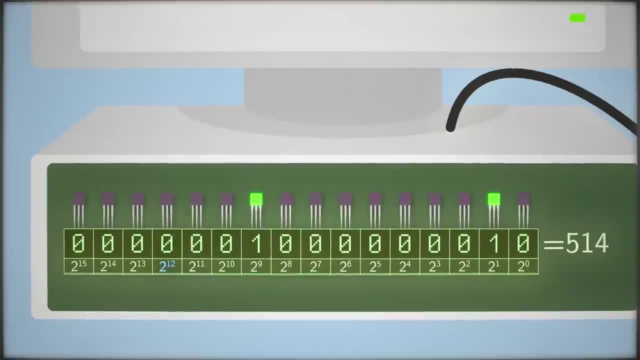 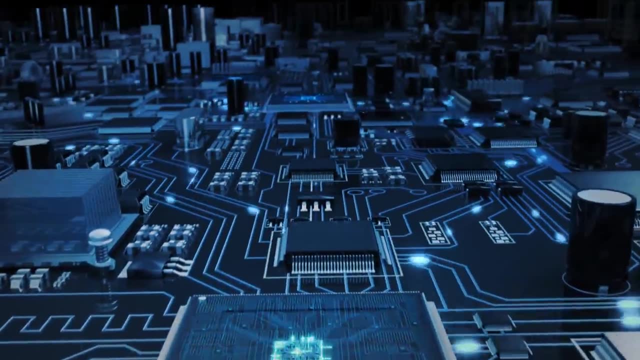 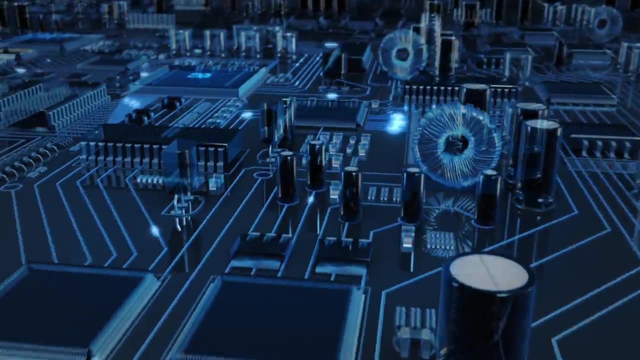 13th bit had to flip from a zero to a one. But why would that happen? Computers work precisely because bits don't flip, unless we want them to, Or do they? Looking into the problem, Belgian investigators found reports of similar issues from big computer companies. 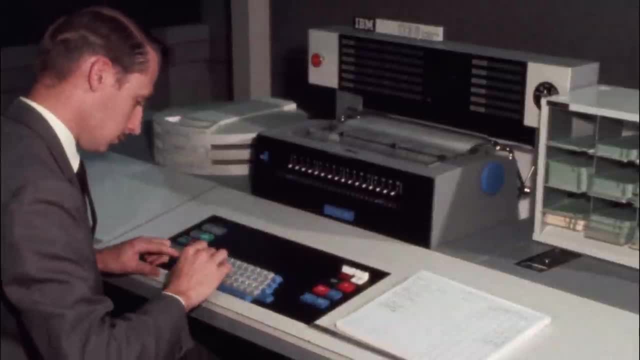 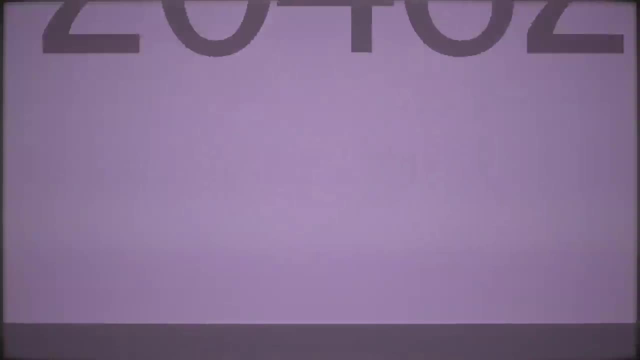 starting in the 1970s. In 1978, Intel reported some strange errors popping up in their 16-kilobit dynamic random atom. This was the first time Intel reported errors in their 16-kilobit dynamic random access memory Ones would spontaneously flip to zeros with no apparent cause. 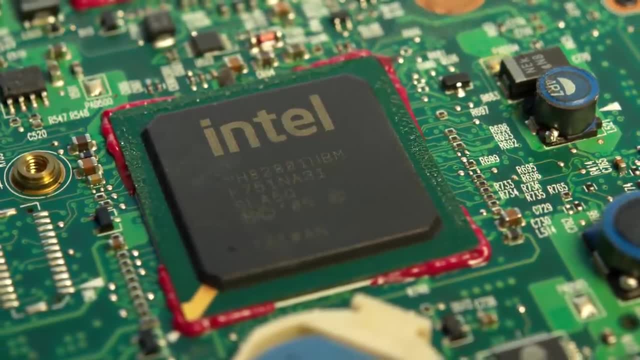 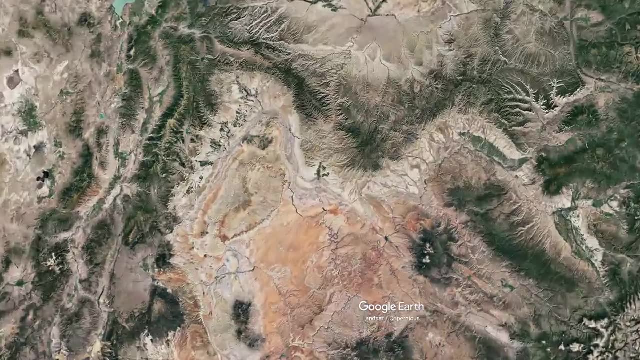 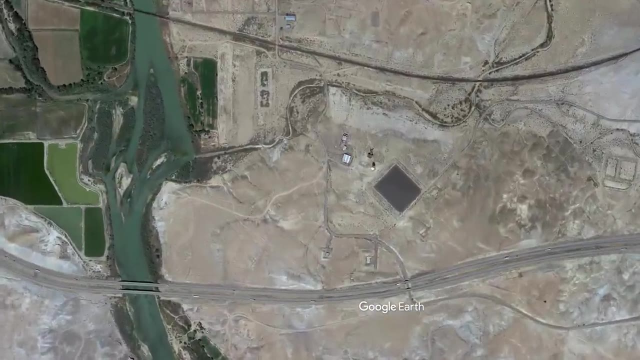 The problem turned out to be the ceramic packaging the chip was encased in. With the demand for semiconductor packaging skyrocketing in the 1970s, a new manufacturing plant was constructed on the Green River in Colorado. Unfortunately, this site happened to be just downstream of an old uranium mill. Radioactive atoms made their way into the river. 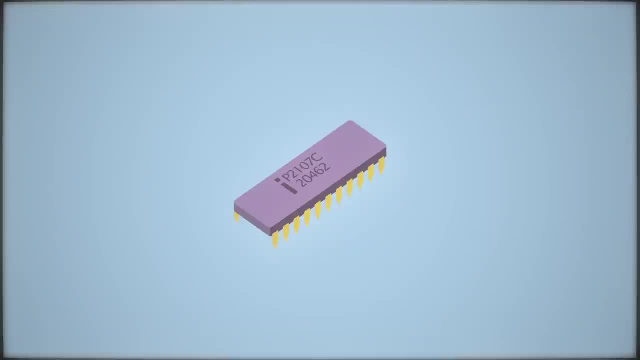 and then into the ceramic packaging for Intel's microchips. Intel's scientists investigating the problem found that even trace amounts of uranium and thorium in the ceramic were sufficient to cause problems In their DRAM. memory was stored as the presence or absence of electrons in a 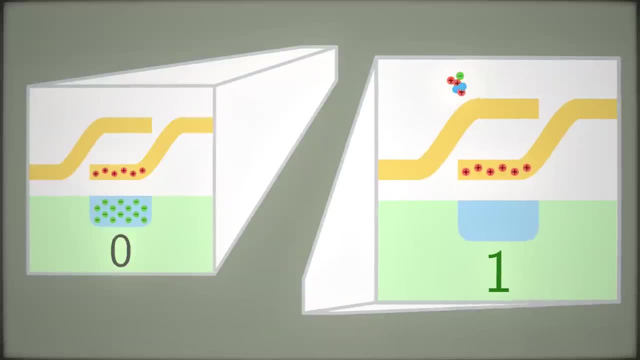 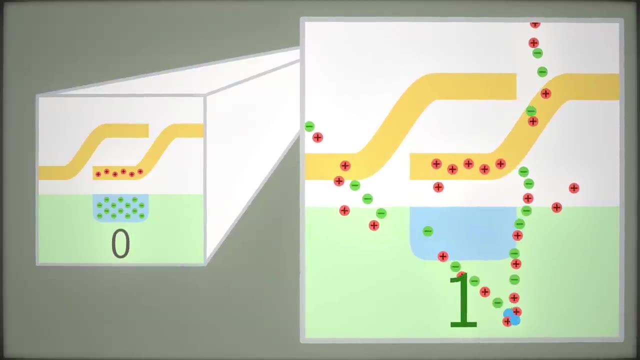 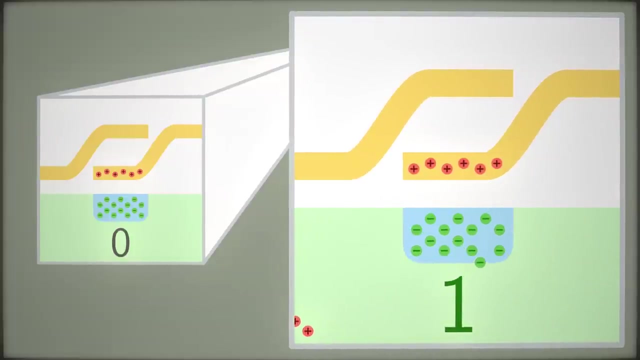 semiconductor. well, The alpha particles emitted by uranium and thorium were energetic and ionizing enough to create electron-hole pairs in the silicon. If an alpha particle struck in just the right place, it could create a large number of free charge carriers, causing electrons to accumulate in the 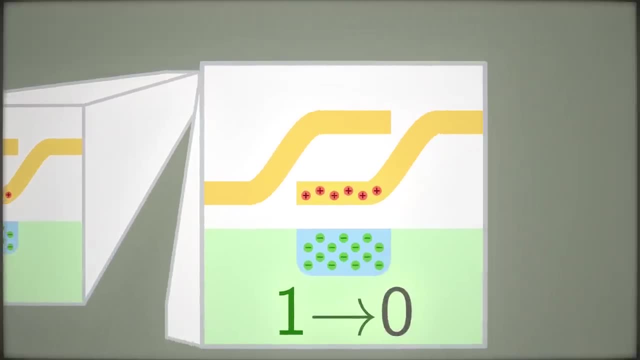 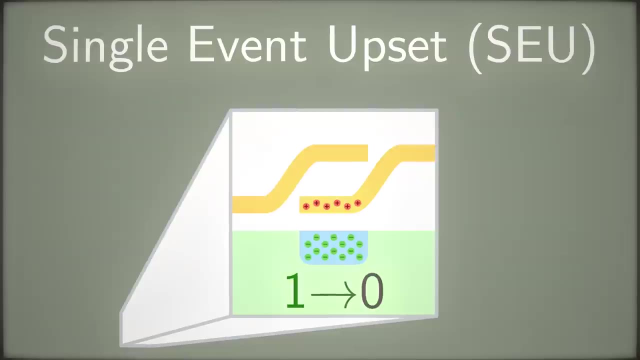 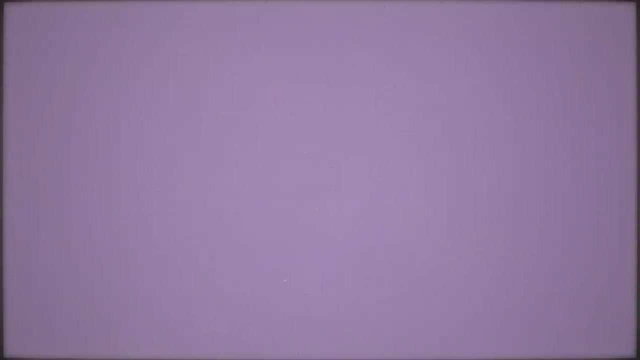 well flipping a 1 to a 0. This is known as a single-event upset, a type of soft error. The error is soft because the device hasn't been damaged. The bit has changed, but you could erase it and rewrite it with no problems. Investigators exposed the chips to alpha emitters with different. 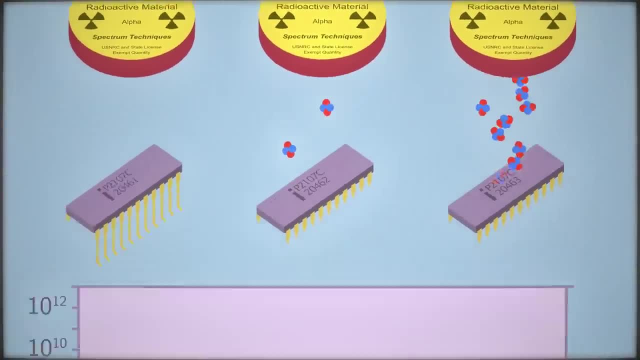 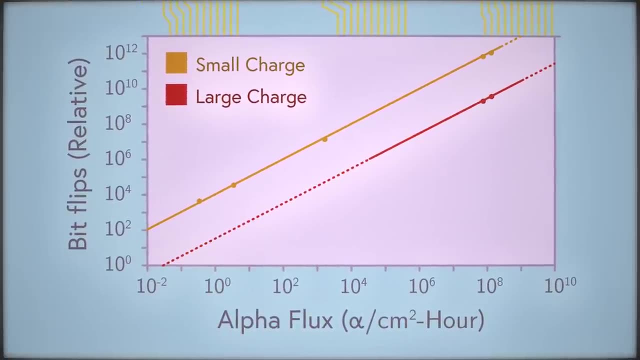 levels of activity. and, just as you'd expect, they found the number of bit flips left on the chip, The number of bit flips directly correlated with the number of alpha particles the chip had been exposed to. The reason this problem was identified in the 1970s was because chip components 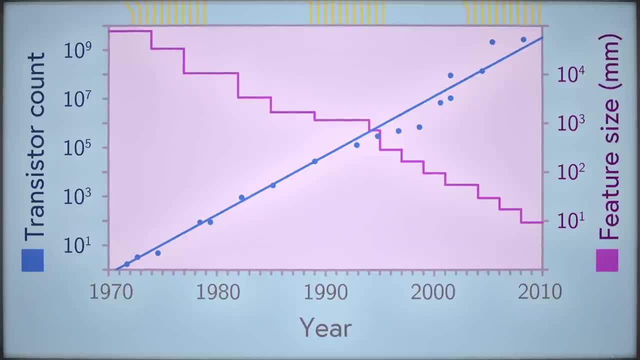 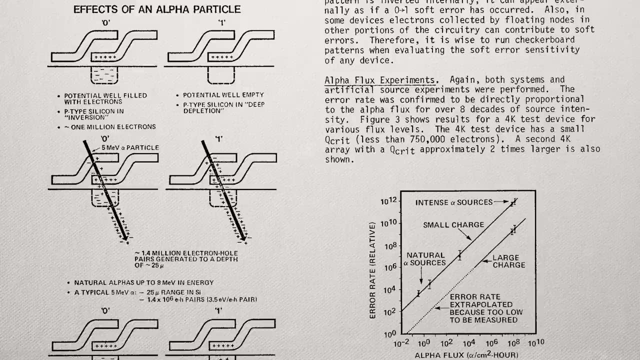 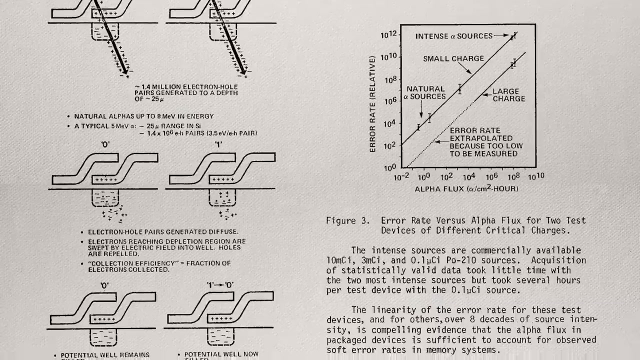 had been miniaturized to the point where a single alpha particle could produce enough charge to flip a bit Immediately. these findings attracted a lot of attention. Before the paper was published, it was widely circulated in the industry And, as a result, chip manufacturers were a lot more careful. 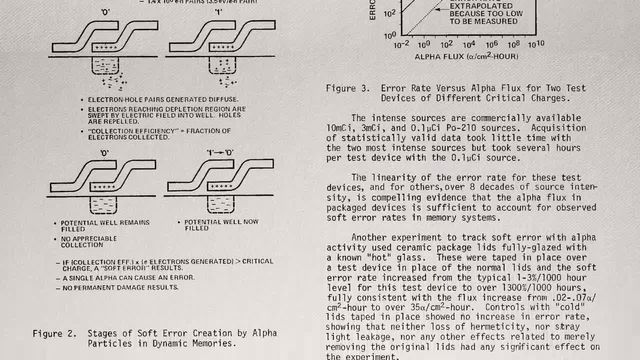 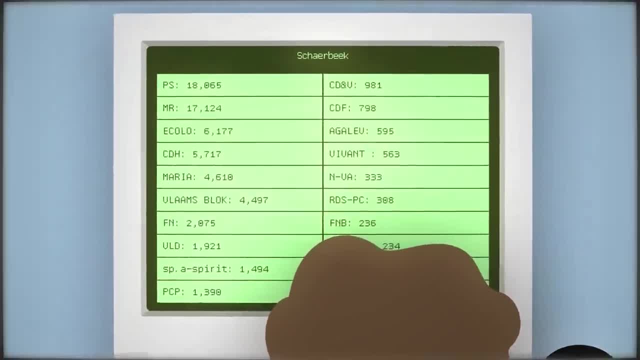 to avoid radioactive materials when producing the chip components. In the 1970s, the chip components produced microchips and packaging. Therefore, the bit flip that gave Maria Windevogel 4096 extra votes wasn't caused by natural radioactivity in the computer. So where did it come from? 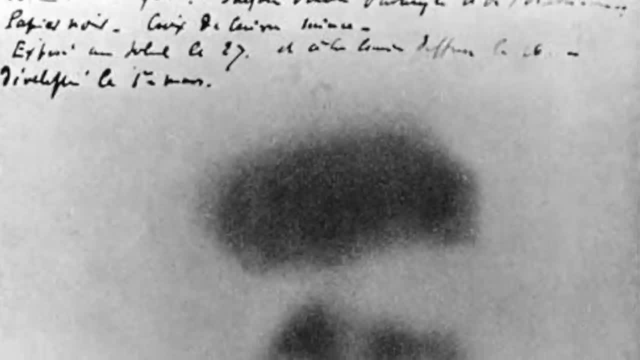 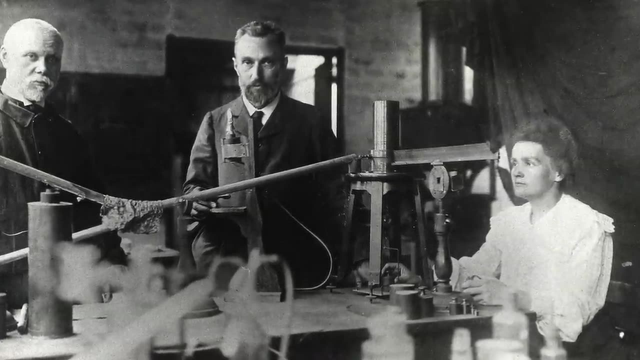 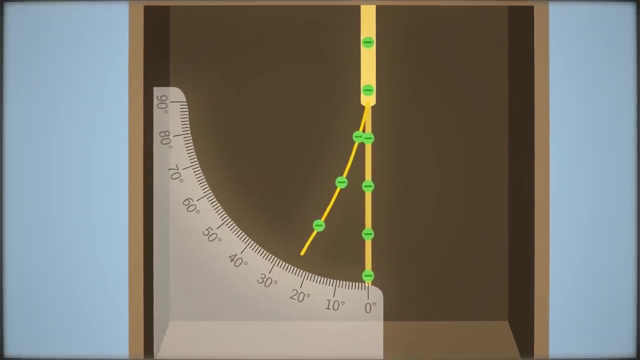 After Henri Becquerel discovered radioactivity with uranium in 1896,, scientists sought a way to measure it: How radioactive were different materials? One way to do this is with a gold leaf electrometer. When it's charged, the leaf is repelled and you can measure the amount of charge by the angle of the leaf. Now, if ionizing radiation 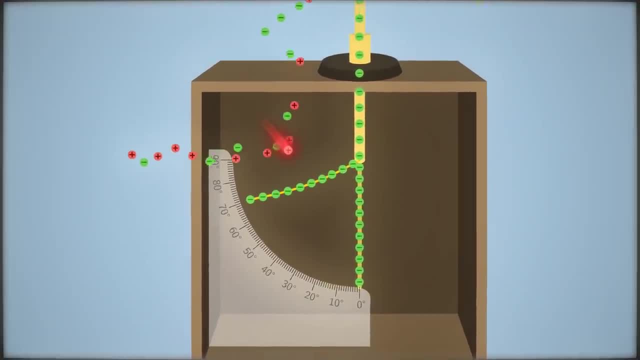 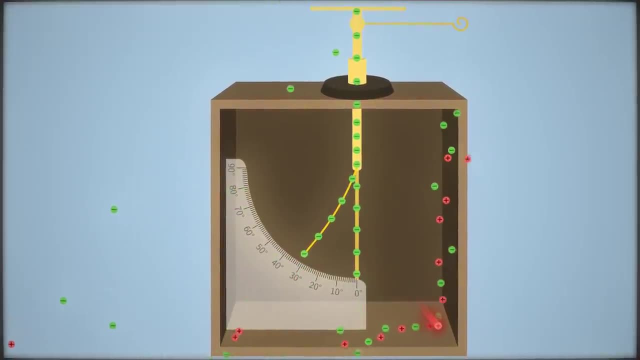 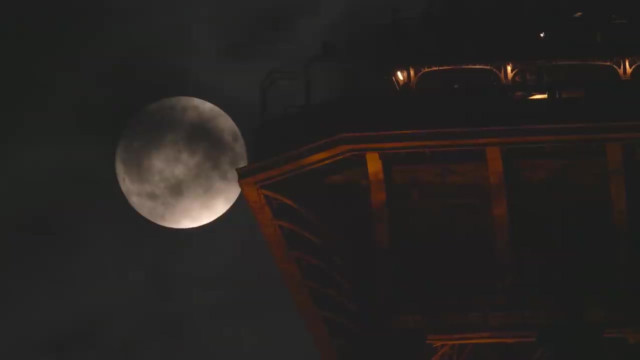 enters the chamber, it rips electrons off air molecules, creating positive and negative charges. Opposite charges are attracted to the leaf, discharging it over time. The higher the level of ionizing radiation, the faster the device discharges. In 1910, Theodor Wolff took his electrometer to the top of the Eiffel Tower, Since radioactivity was 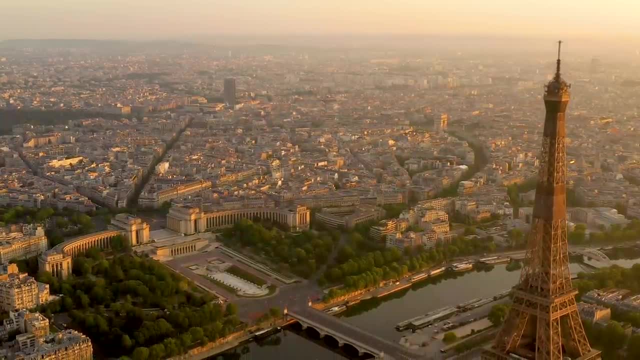 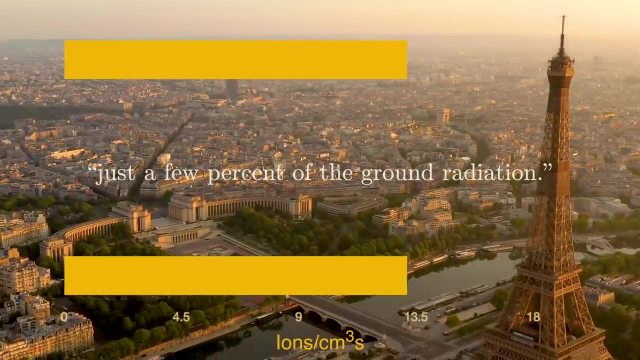 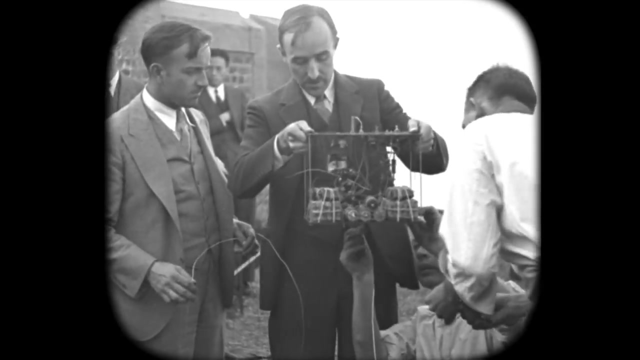 found in the soil and rocks of Earth. he expected that 300 meters up the radiation would be just a few percent of the ground radiation. Instead he found only a slight decrease. In 1911, Austrian physicist Victor Hess decided to take this experiment further. 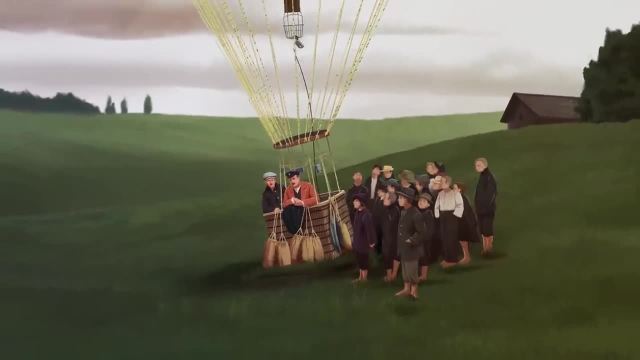 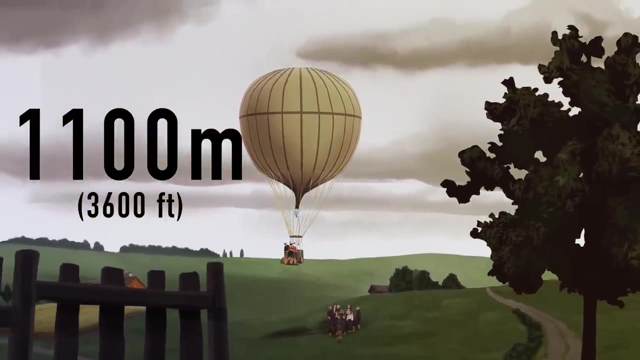 Literally, He loaded electroscopes into the basket of a hydrogen balloon. In his first two flights he observed the same thing as Wolff: Up to an altitude of 1100 meters revealed no fundamental change in radiation compared to the values observed on the ground. 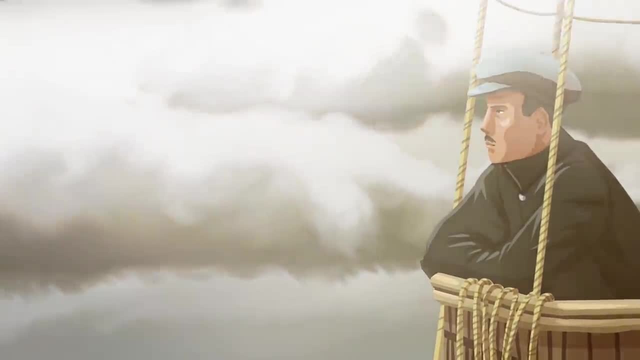 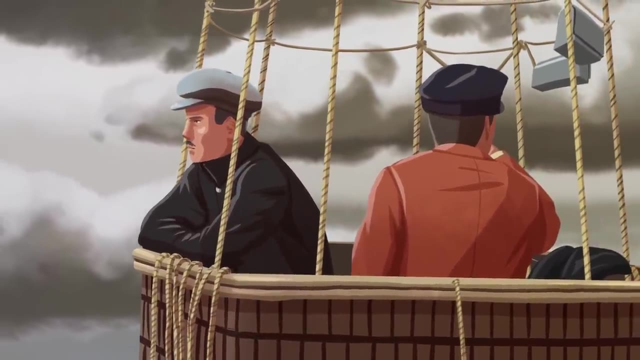 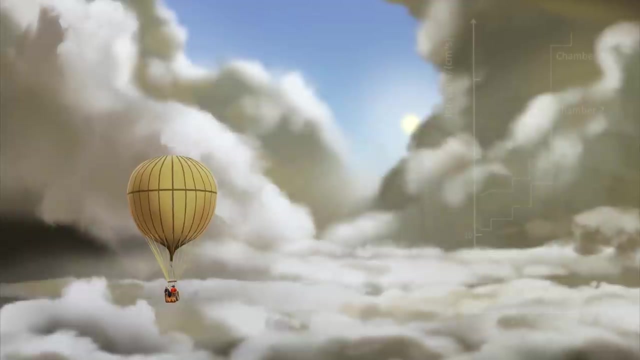 But the next year he conducted seven balloon flights up to an altitude of 5200 meters. And here he discovered something remarkable: While there was an initial drop in radiation for the first several hundred meters above one kilometer or so the level, 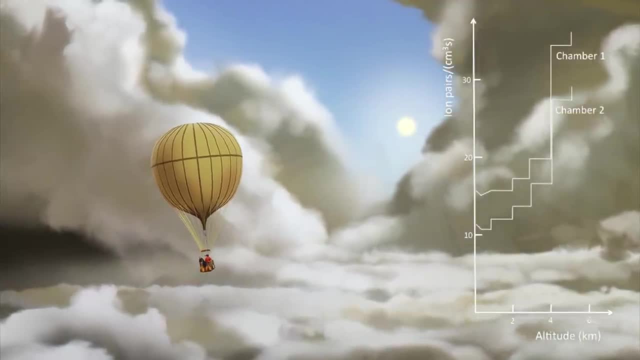 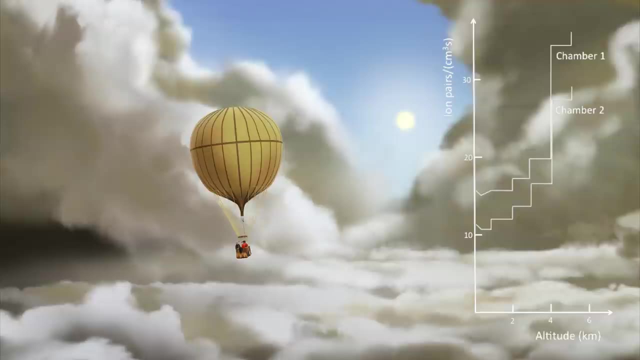 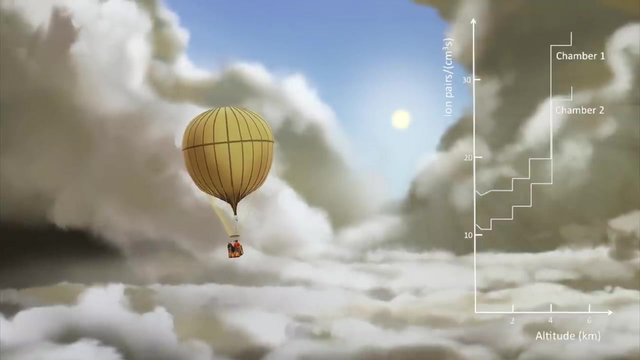 increased with increasing altitude. At his maximum height, the level of radiation was several times greater than it was on the ground. The radiation appeared to be coming not from the Earth but from the sky. Hess scheduled one of his balloon flights during a solar eclipse. 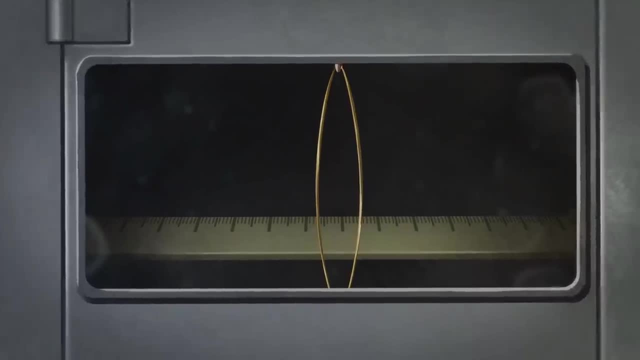 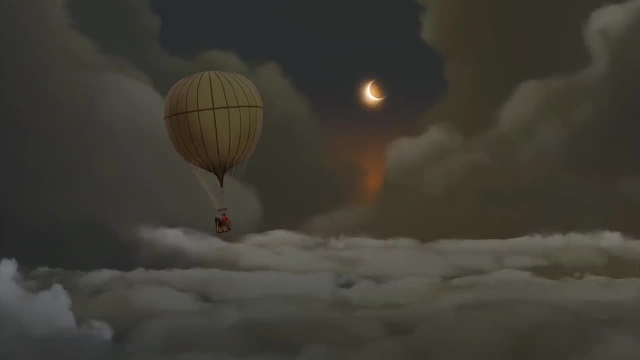 and as the moon passed in front of the sun, he carefully watched his instruments, But the readings were unaffected. Even with the sun half covered, the level of radiation was the same, Since no influence of the eclipse on the penetrating radiation was noted. 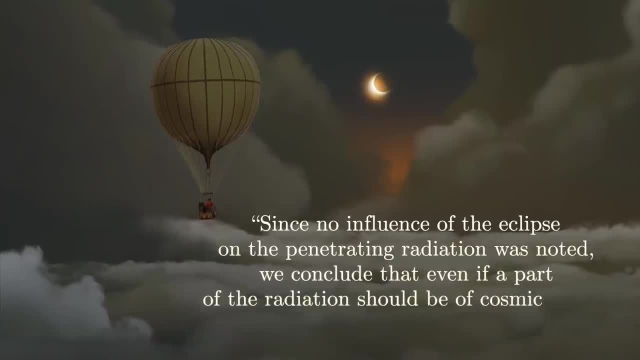 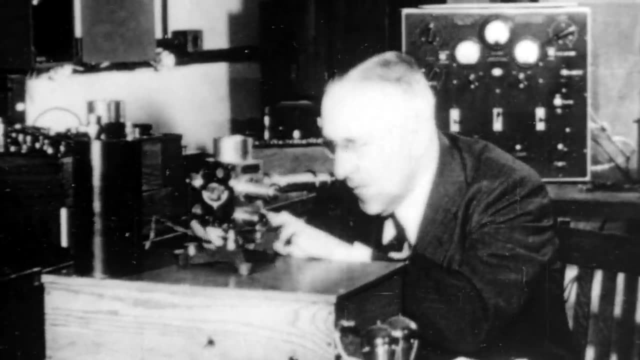 we conclude that even if a part of the radiation should be of cosmic origin, it hardly emanates from the sun. Victor Hess had discovered cosmic rays- high-energy radiation from space. But what were these rays exactly and where were they coming from? 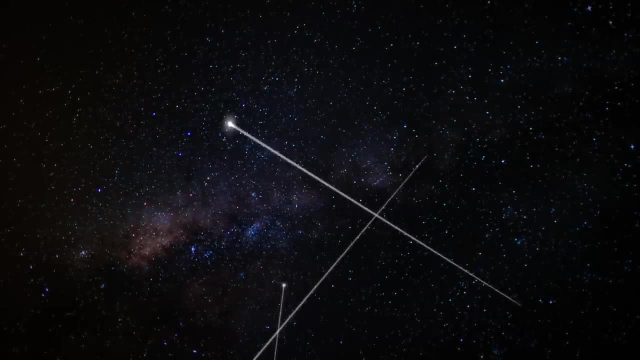 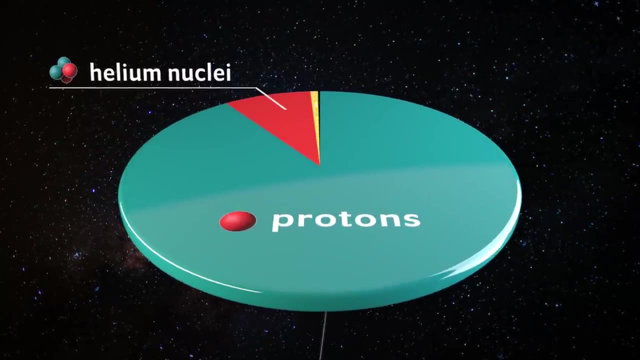 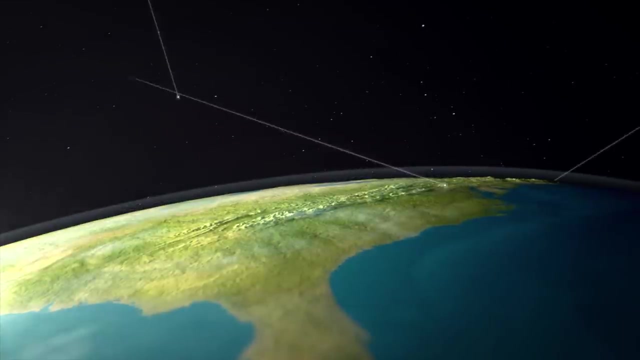 Well, today we know they aren't electromagnetic rays, as many suspected, but particles. Around 90% are protons, 9% are helium nuclei and 1% are heavy-duty particles. Some of them are from the sun, but they have comparatively low energy, High-energy cosmic 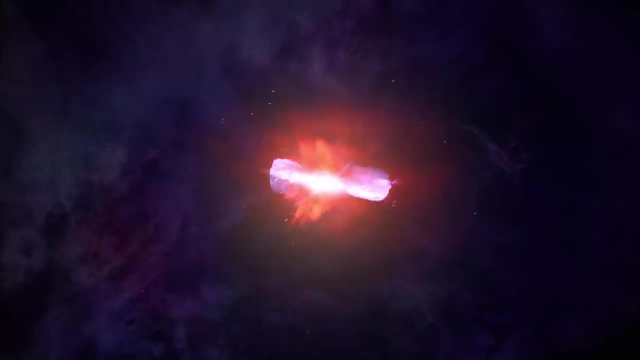 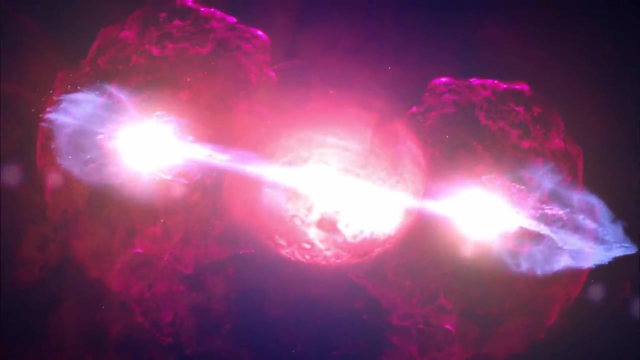 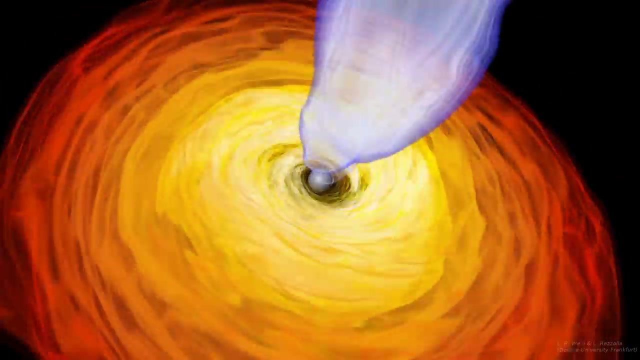 rays moving very close to the speed of light come from exploding stars, supernovae in our own galaxy and in others, And the highest energy particles are thought to come from black holes, including the supermassive black holes at the centers of galaxies, But it's hard to pin down exactly where. 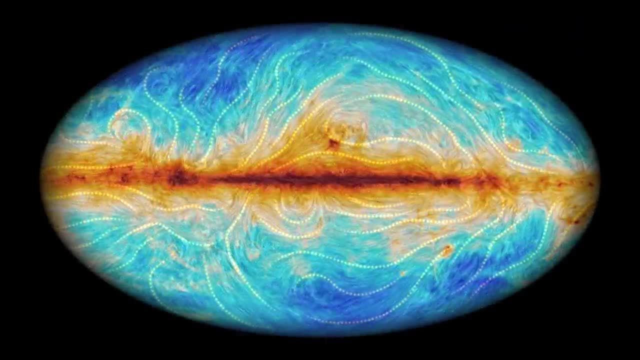 cosmic rays come from, because they don't come from the center of the galaxy. They come from the center of the universe. As charged particles, they're deflected by magnetic fields in space, so they can wind their way through the universe for billions of years. 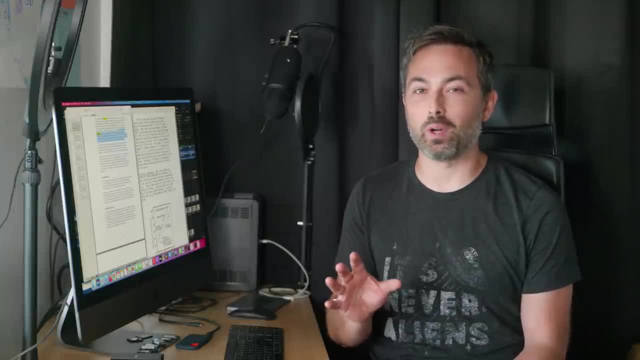 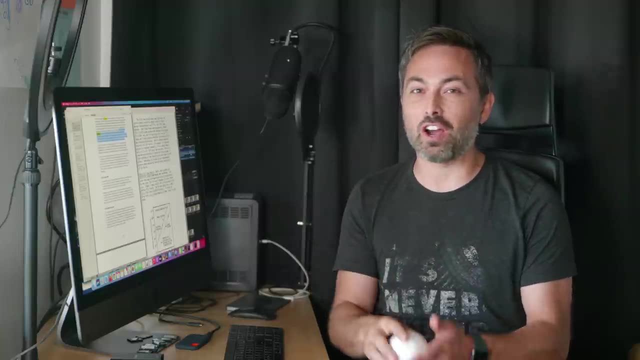 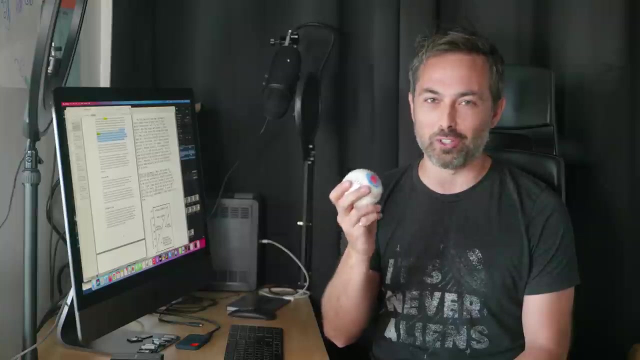 A cosmic ray detected on October 15th 1991, had an energy of 51 joules, That is a single subatomic particle with the energy of a baseball going 100 kilometers per hour. For obvious reasons it was dubbed the OMG particle. But primary cosmic rays like these 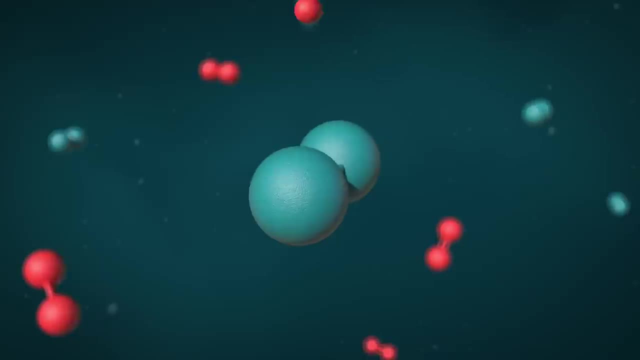 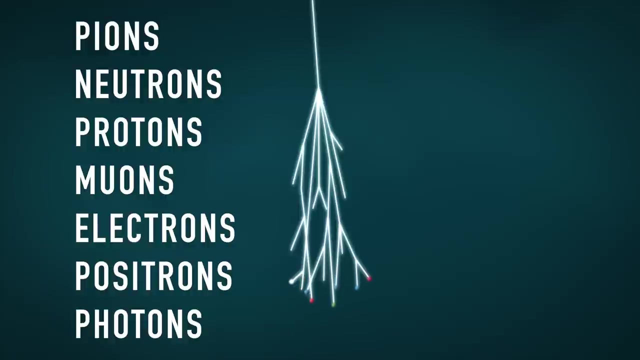 don't make it down to Earth's surface. Instead, they collide with air molecules around 25 kilometers above the ground and create new particles like pions. These collide and decay into other particles like neutrons, protons, muons, electrons, positrons and photons. 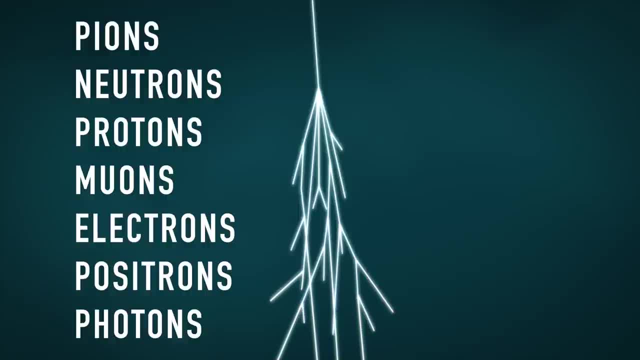 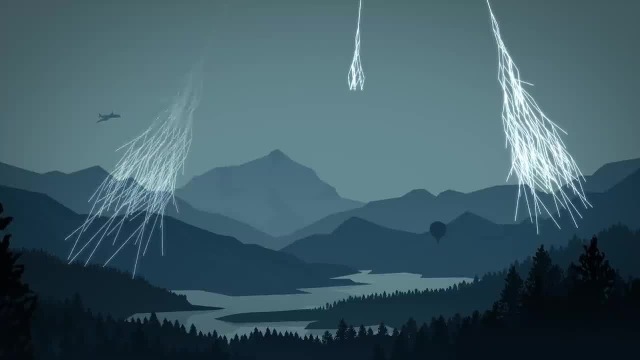 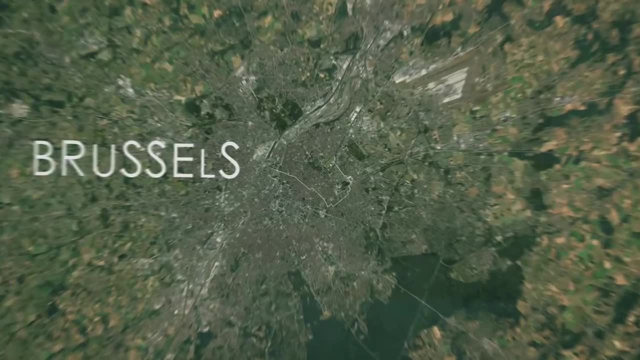 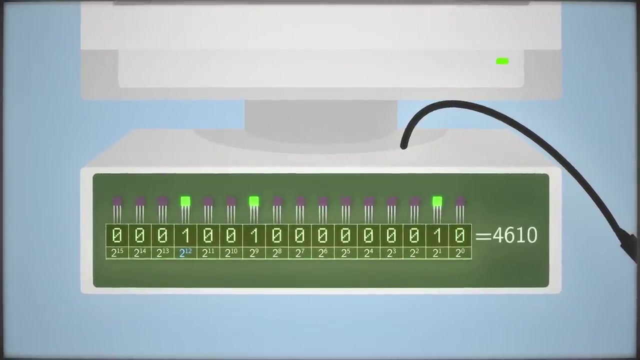 which in turn collide with other air molecules in one long cascade. So from a single primary cosmic ray comes a shower of particles streaming towards the Earth. It is one of these particles that investigators suspect struck a transistor in a computer in Belgium, flipping the 13th bit from a zero to a one and giving Maria Windevogel 4,096 extra votes. 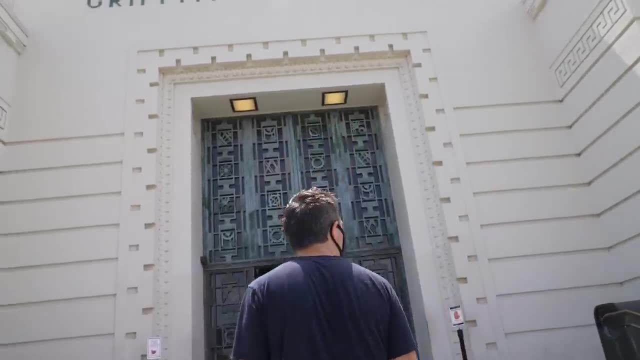 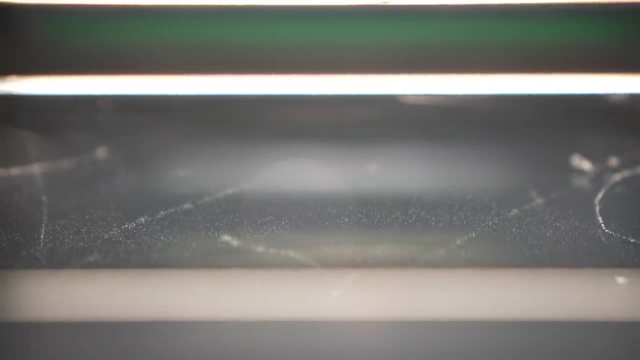 But how often do things like this happen? In 1911, Charles Wilson made it possible to see the cosmic rays all around us when he perfected his cloud chamber, an enclosure with supersaturated water or alcohol vapor. This was the first time the cosmic rays had been seen in the atmosphere. 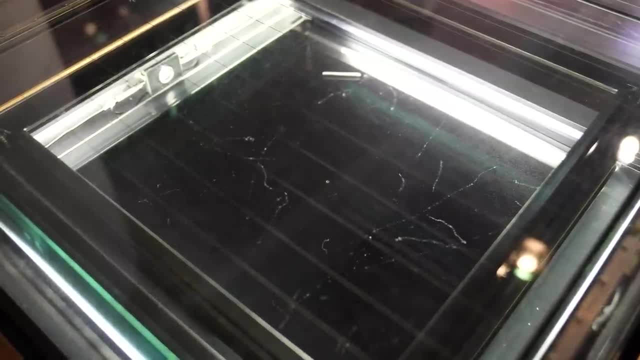 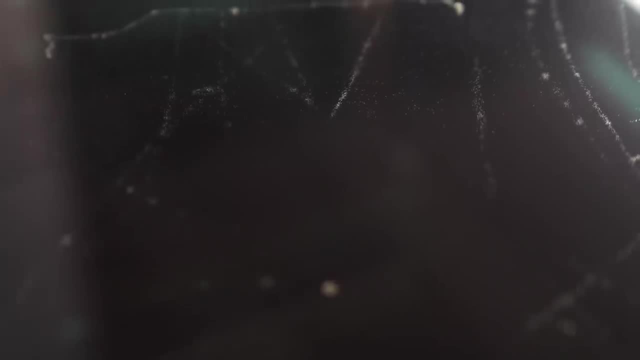 When a cosmic ray passes through the chamber, it ionizes the gas, causing vapor to condense into tiny droplets on the ions revealing the path of the particle. Alpha particles helium nuclei leave short, thick tracks, while beta particles, electrons. 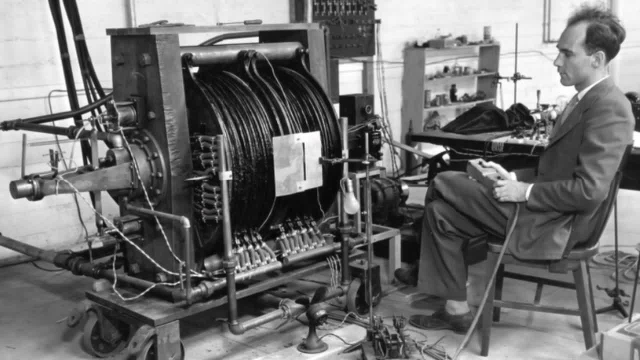 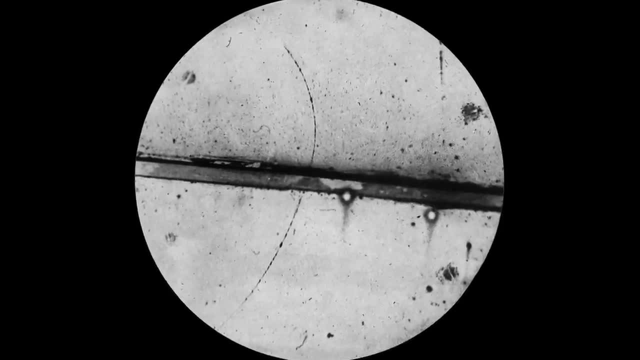 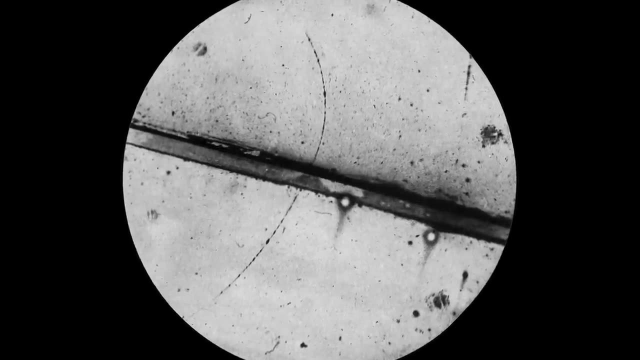 leave long skinny trails. In 1932, Carl Anderson identified a trail that looked like it was made by an electron, but in the applied magnetic field it curved in the wrong direction, implying it had a positive charge. Anderson had found the antielectron or positron. It was the first confirmed sighting. 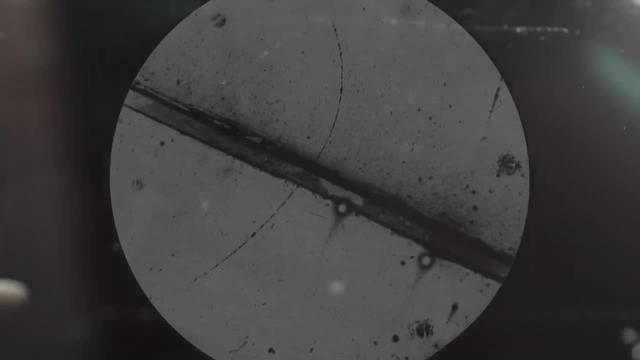 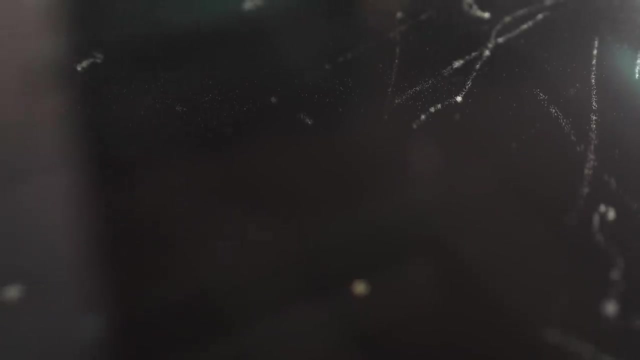 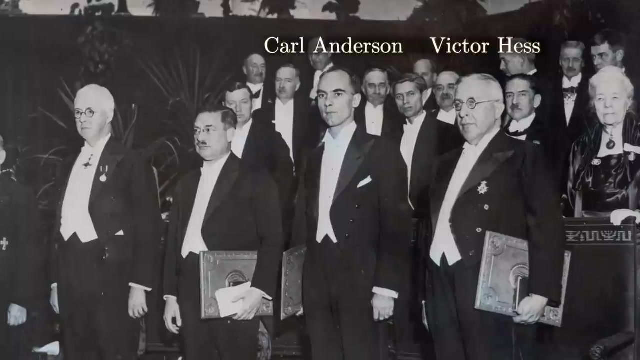 of antimatter. Four years later, also using a cloud chamber, he discovered the muon, again in cosmic rays. For his discovery of the positron, Anderson was awarded the Nobel Prize in Physics in 1936. He shared the prize with Victor Hess, the man who discovered cosmic. 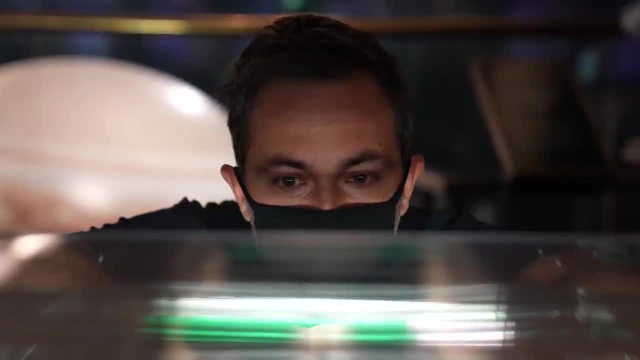 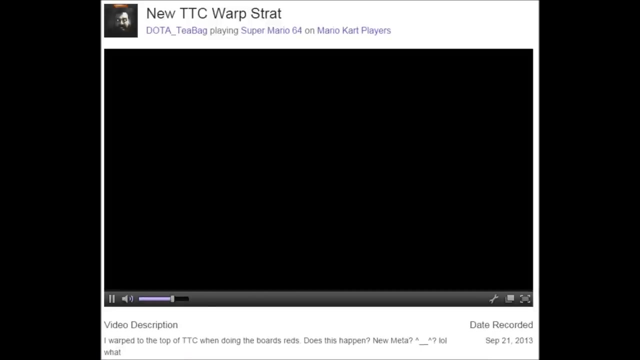 rays in the first place. Invisible particles that affect the cosmic rays, the muon and the positron, were the first to discover the positron. In 1936, Anderson was awarded the Nobel Prize in Physics. This is possibly the rarest thing to ever happen in a video game In 2013,. user: DotaTbag. 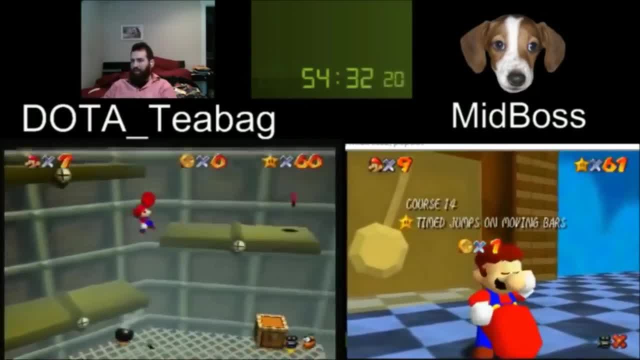 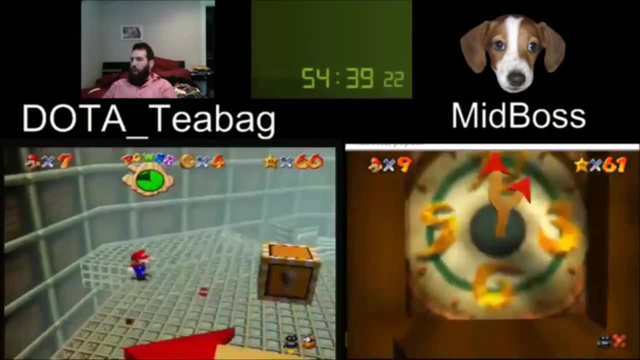 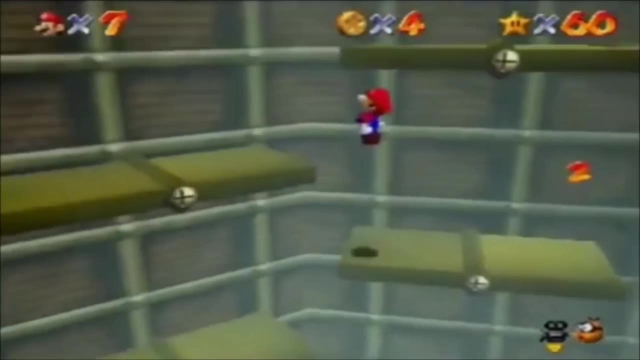 was speedrunning Super Mario 64 on the console In the level TikTok Clock, he suddenly up-warps onto a higher platform. The move shaves off a few seconds and it seems like a newly discovered glitch in the game that could give speedrunners. 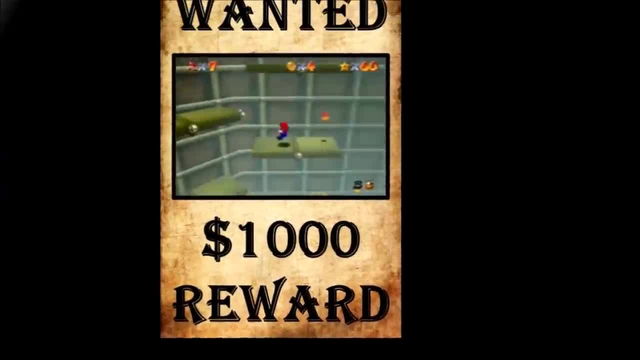 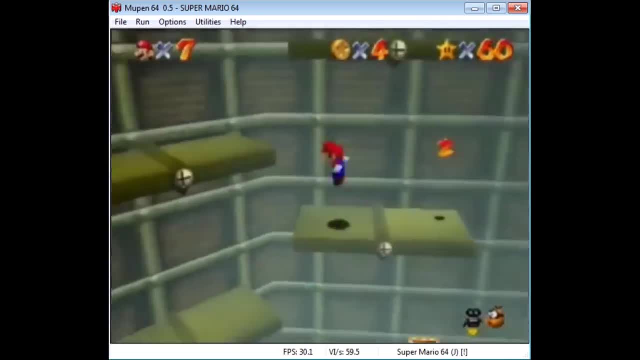 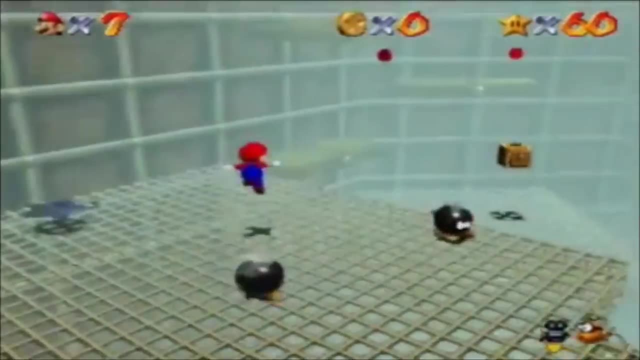 an edge. User Pannenkoek12 put out a $1,000 bounty for anyone who could replicate the up-warp, But so far, after six years, no one has been able to. The best explanation anyone can come up with is that a cosmic ray caused the glitch. It's been shown that a single bitflip in the first 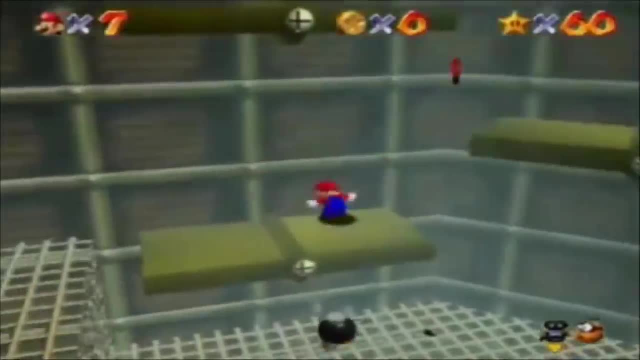 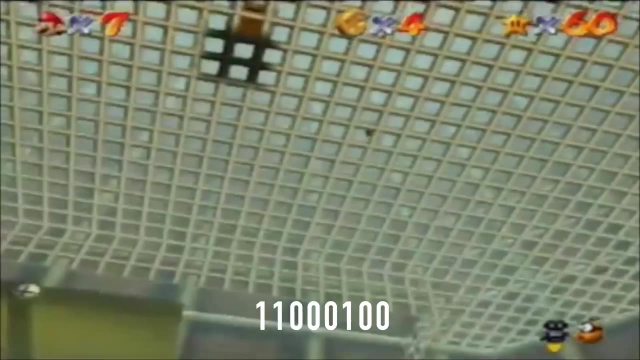 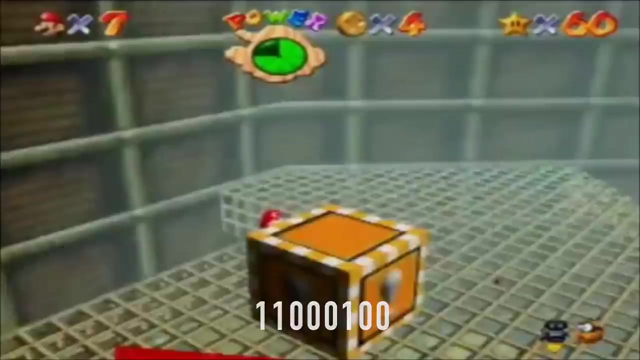 byte of Mario's height coordinate could have caused the effect. On the main level it was 11000101.. But if you flip the last one to a zero, it changes his vertical position And just by chance this new height coincides with the higher floor. Pannenkoek12 wrote a. 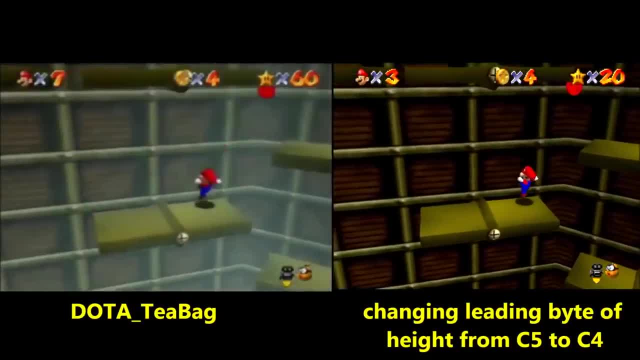 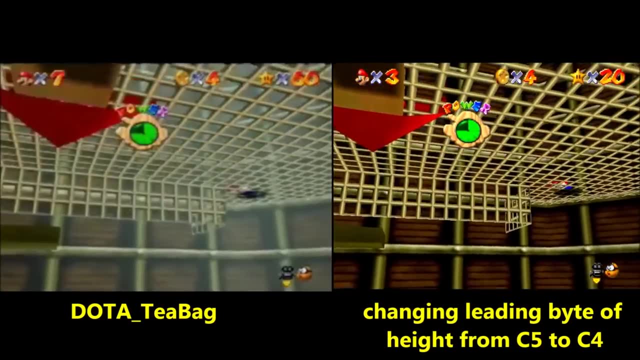 script to manually flip the bit at the right moment and was able to achieve the same up-warp. This is a particularly visible bitflip, but the truth is cosmic rays are triggering bitflips all the time. An upset there, a transient there. 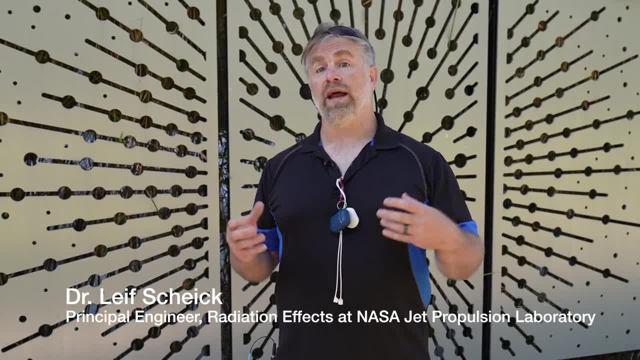 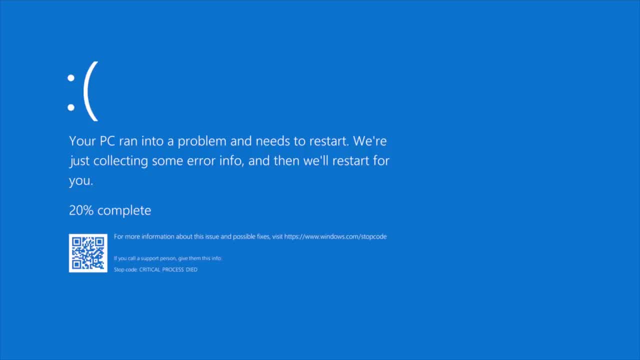 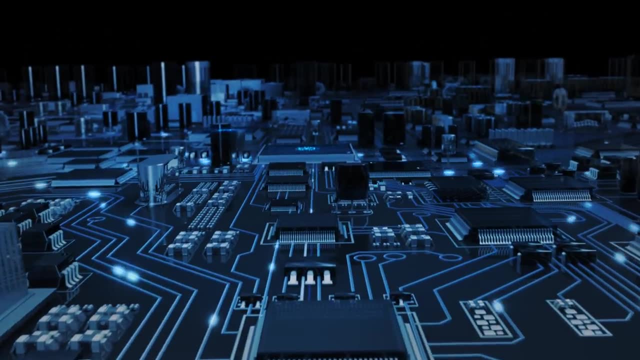 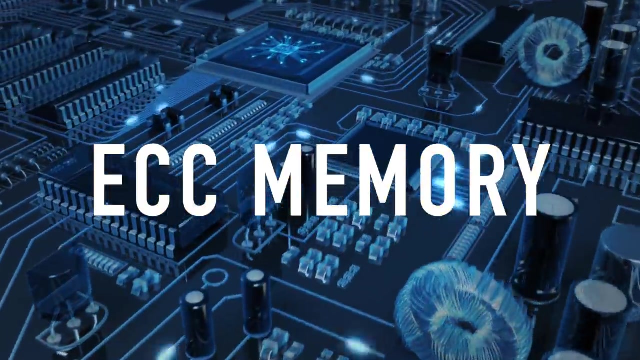 can all think of it as a bitflip. These days there are a number of ways computer chips are made resilient in the face of bitflips, like error correction code or ECC memory. But you can't totally prevent bitflips from happening. 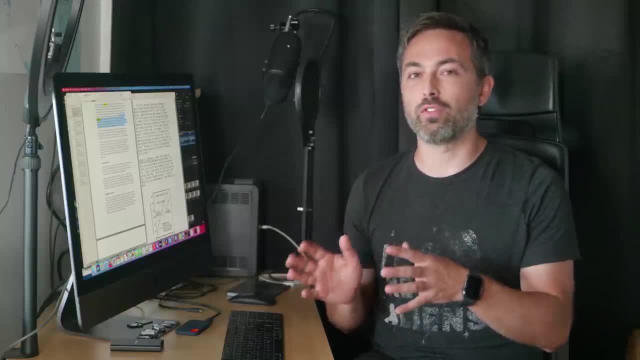 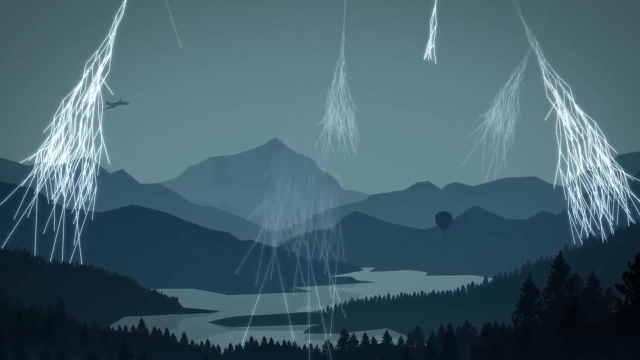 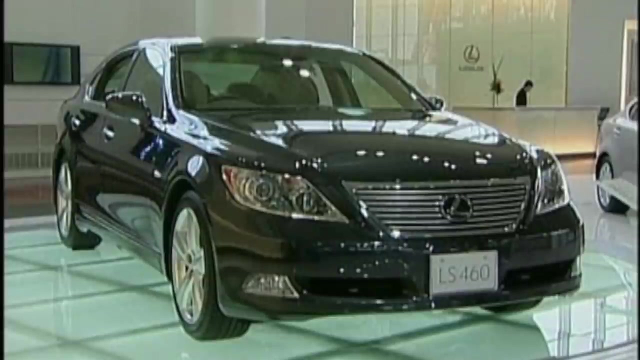 In 1996, IBM estimated that, for each 256 megabytes of RAM, one bitflip occurs per month, And the main culprit seems to be neutrons created in the shower of particles from cosmic rays. Starting in 2009,, Toyota recalled millions of vehicles due to the problem of 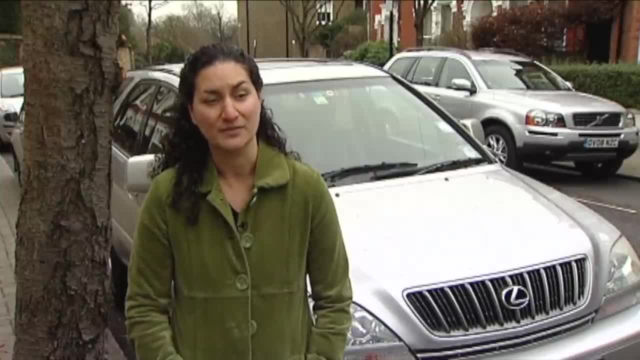 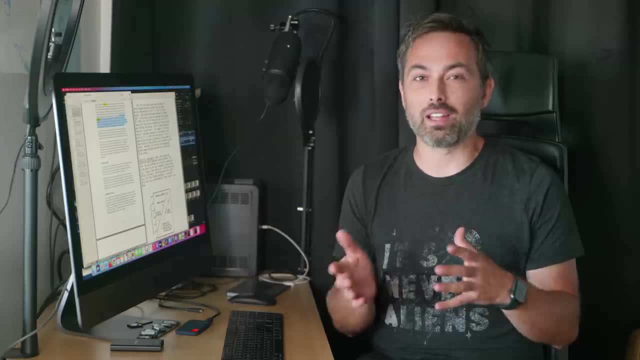 unintended acceleration. We were in the fast lane, driving at about 70, and he said that the car was continuing to accelerate And he couldn't bring it to a stop. Many speculated that cosmic ray induced bits of the ray were likely the cause of the problem. 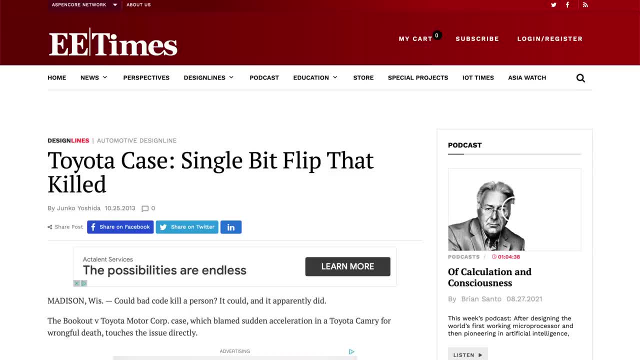 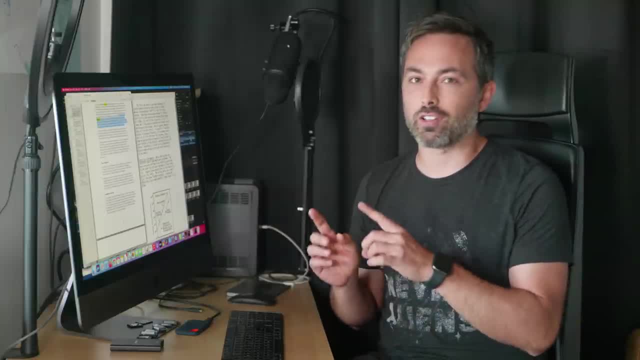 So we're not sure. if that's the case, We're just hoping that there are other ways of doing the same thing. flips in the electronic control system were the cause, So much so that NASA was called in to help with the investigation. But it turns out cosmic rays were probably not the culprit NASA identified. 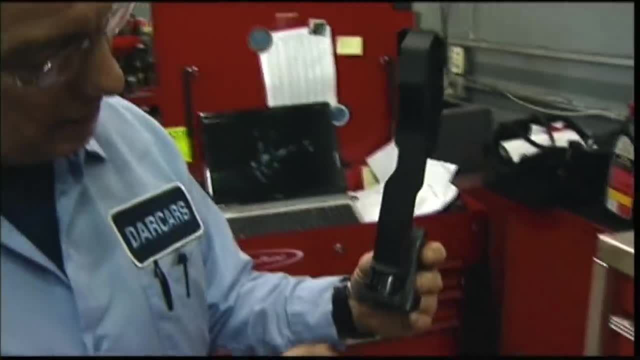 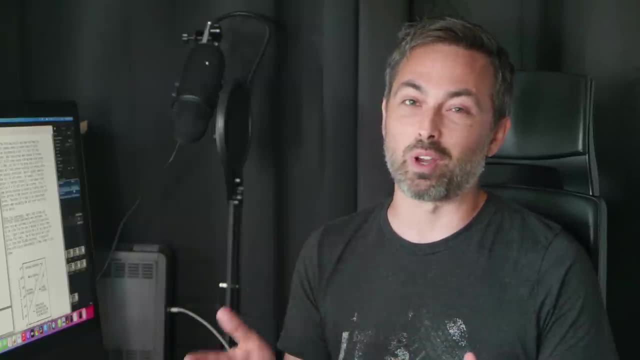 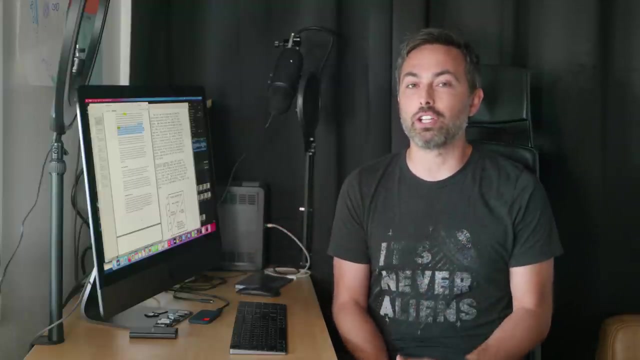 as the main causes: sticky accelerator pedals, poorly fitted floor mats and, most commonly, drivers pushing on the accelerator thinking it was the brake. But cosmic rays have caused crashes of supercomputers, especially at higher elevations. Los Alamos National Labs, located 2200 meters, above sea level is constantly dealing with neutron-induced supercomputer crashes, So the software autosaves frequently and neutron detectors have been installed throughout the facility. If you go even higher, like climbing up to cruising altitude in a plane, you can see the radiation from cosmic rays increasing on a Geiger counter. To 0.5 microsieverts per hour at 18,000 feet, up to 1 microsievert per hour at 23,000 feet, over 2 microsieverts per hour at 33,000 feet and over 3 microsieverts per hour at even higher altitudes and towards the poles. 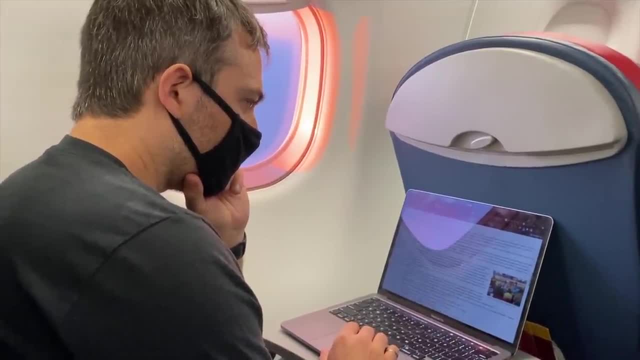 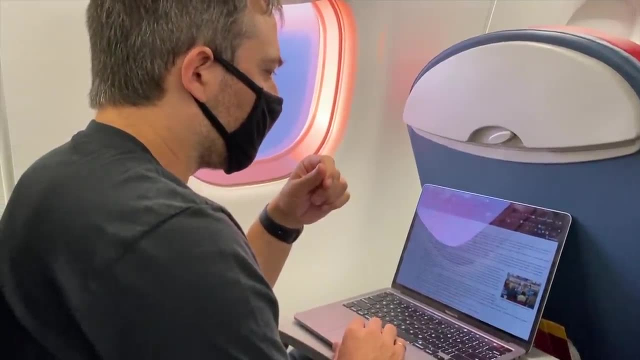 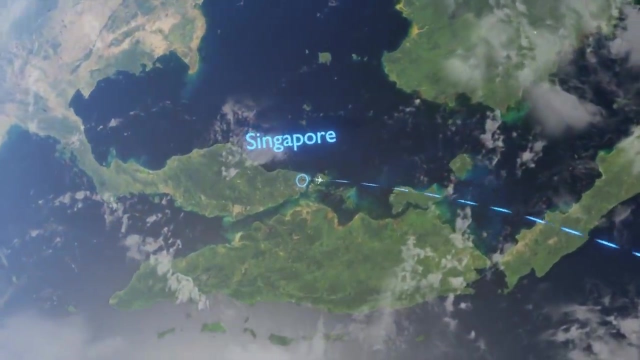 At cruising altitude. this increases the chance of a single event upset by 10 to 30 times. This isn't critical if it happens in your laptop, but what if it occurs in the flight computer? On October 7th 2008,, an Airbus A330 took off from Singapore to Perth. 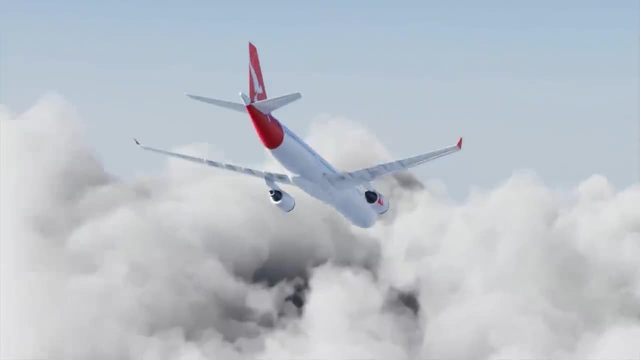 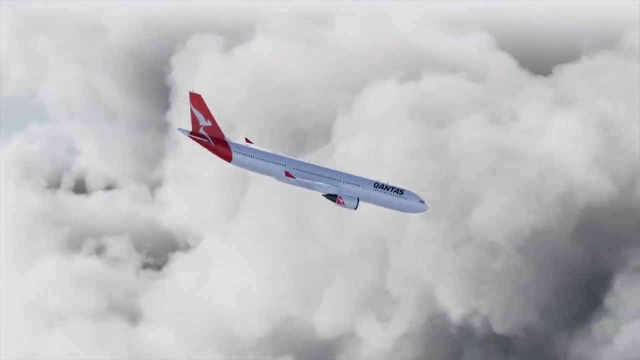 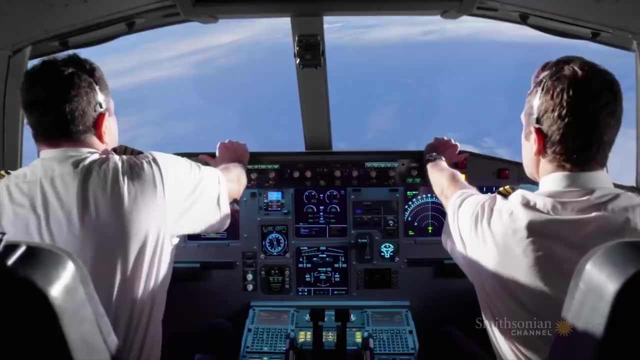 Just over three hours into the flight, the plane suddenly pitched down, diving 200 meters in 20 seconds. Inside the plane, everyone experienced negative 0.8 g's of acceleration. It would have felt like the plane had flipped over. The g-force was enough even with our three-point harness. 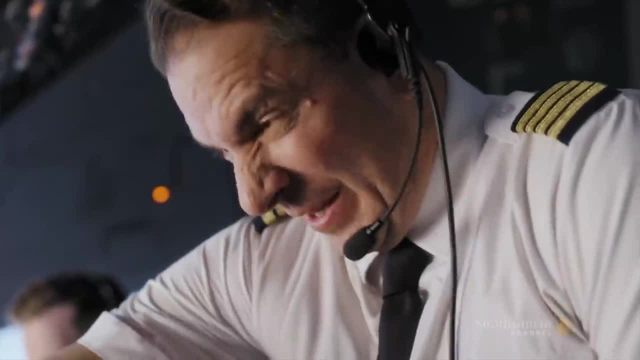 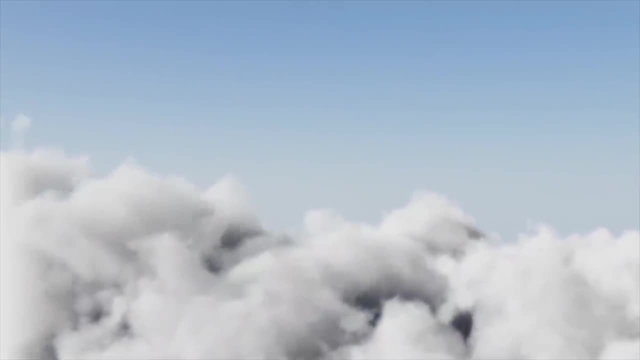 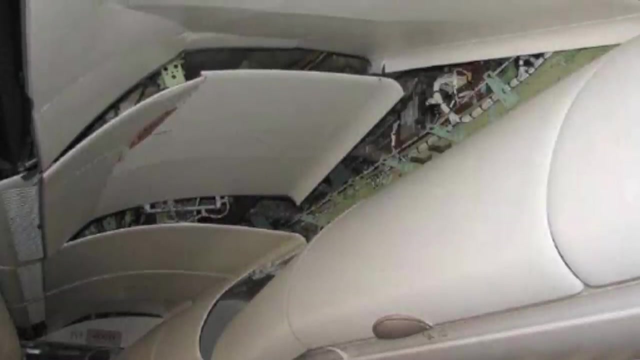 to lift us both out of the seat and push us forward as well. Minutes later, the plane dropped another 120 meters. 119 people on board were injured, many from bumping their heads into the ceiling. So the pilots decided to make an emergency landing in Learmonth. 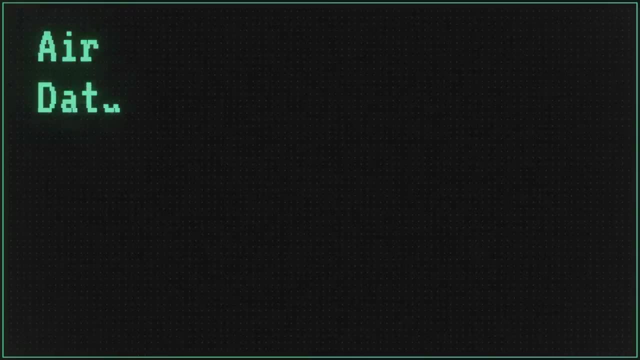 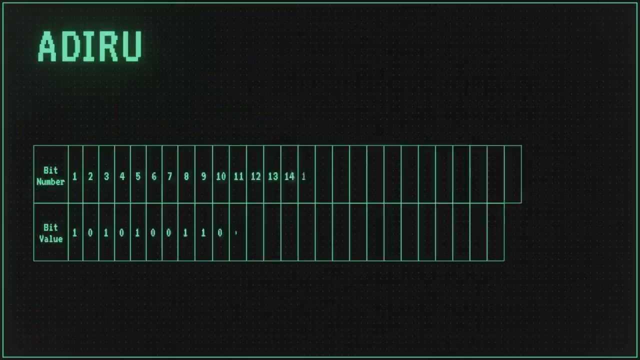 In the investigation that followed, the fault seemed to occur with the first Air Data Inertial Reference Unit, or ADARU for short. This computer supplies critical data like airspeed, angle of attack and altitude. The way it supplies each of these pieces of information is in a 32-bit binary word. The first 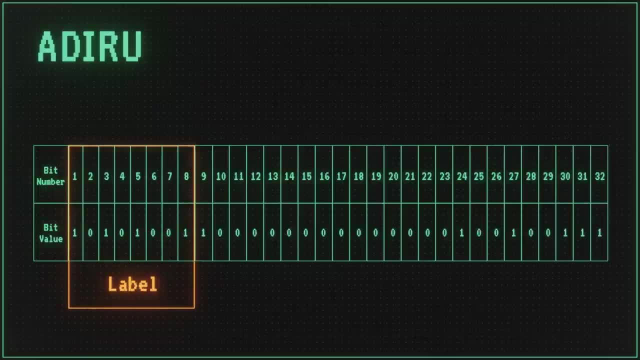 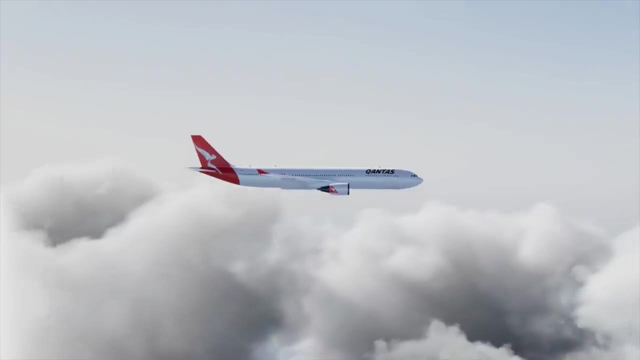 8 bits identify the type of information and bits 11 to 29 encode the actual data. What seems to have happened is that a bit flip in the first 8 bits meant altitude information was mislabeled as angle of attack information. Inside the cockpit alarms went on for overspeed. 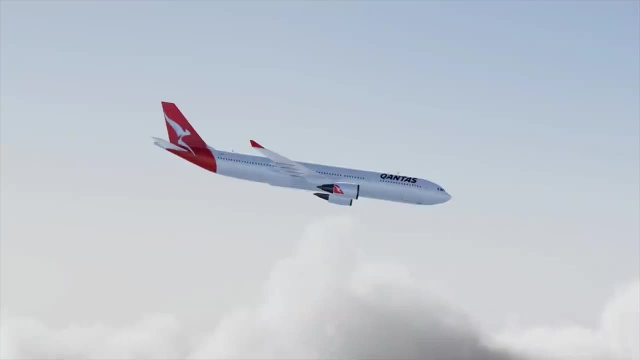 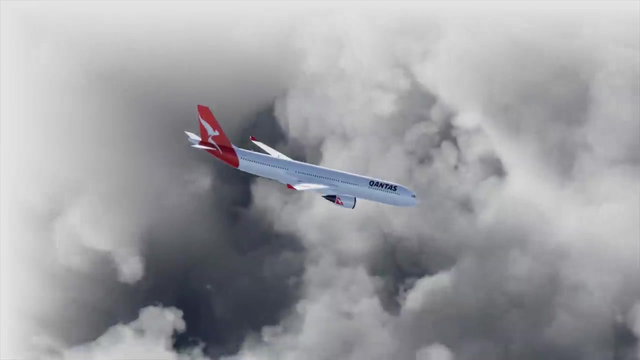 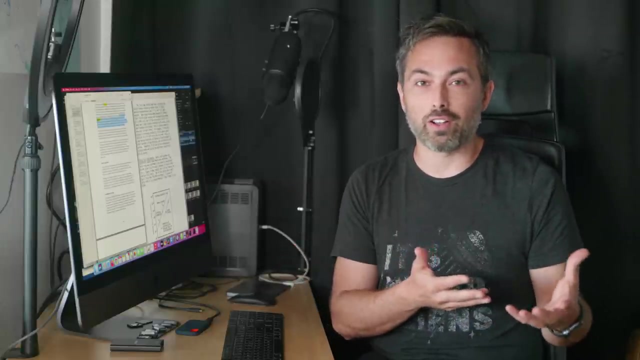 and stall simultaneously- something that should be impossible, But the plane nosed down sharply to correct what it thought was a stall, throwing passengers and crew into the ceiling. Investigators looked into software bugs, software corruption, a hardware fail, physical environment factors and electromagnetic interference. 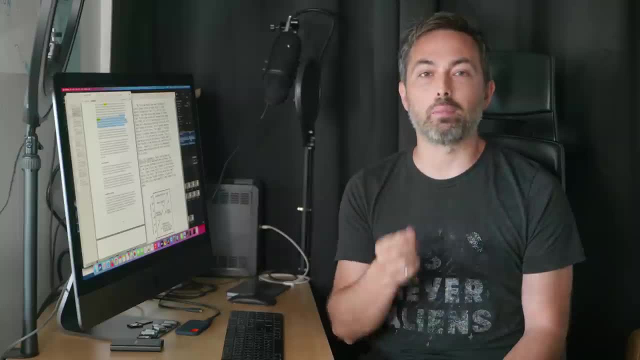 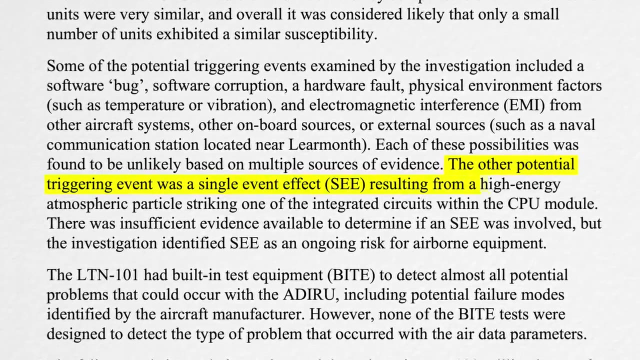 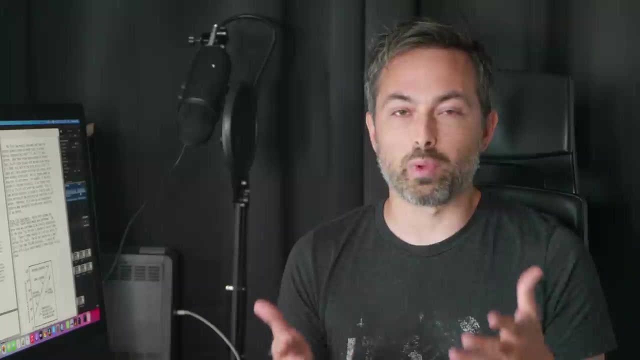 But each of these possibilities was found to be unlikely based on multiple sources of evidence. The other potential triggering event was a single event effect resulting from a high energy atmospheric particle striking one of the integrated circuits within the CPU module. One of the challenges with single event effects is that they can't be triggered by a single event. 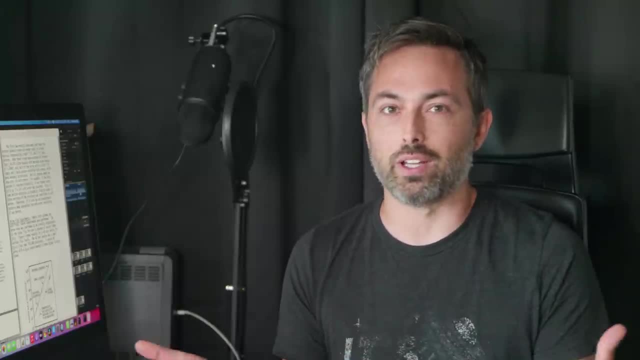 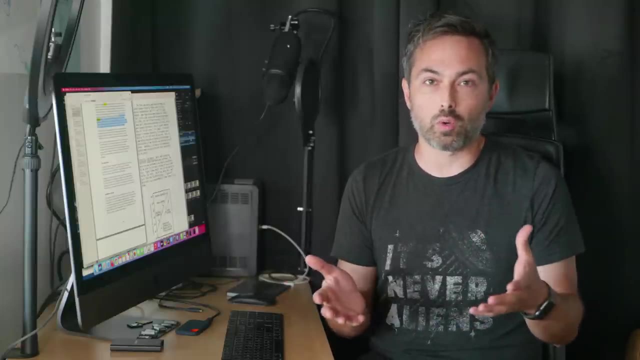 One of the reasons a single event upsets is that they are soft errors: they don't leave a trace. But interestingly, the Airbus A330 was built in 1992 when there were no specific regulatory or aircraft manufacturer requirements for airborne systems to be resilient to single event effects. 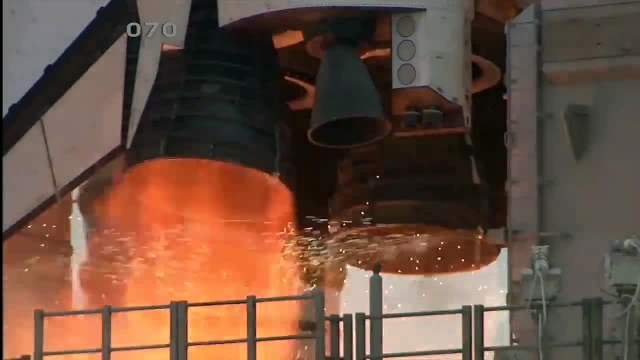 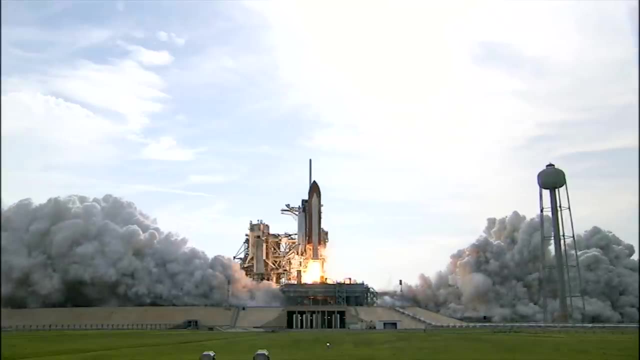 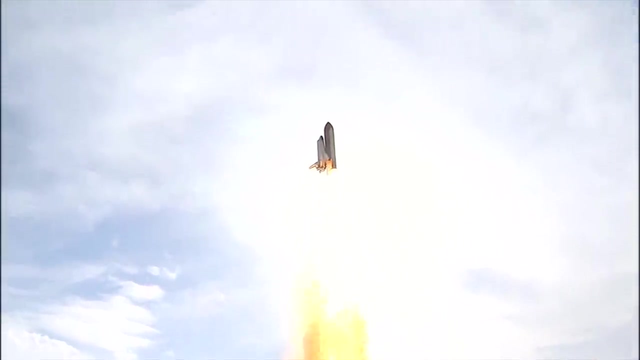 With the Space Shuttle, redundancy was built in from the start For navigation and control. there were four computers simultaneously running identical software. If one computer had a soft, the other three would overrule it and using this setup, they could also track the frequency of bit flips. On one five-day mission- STS-48,, there were 161. 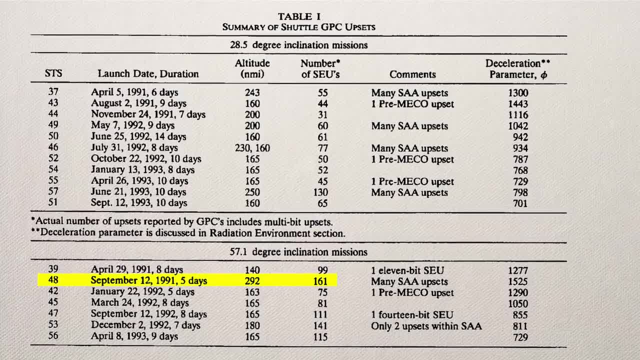 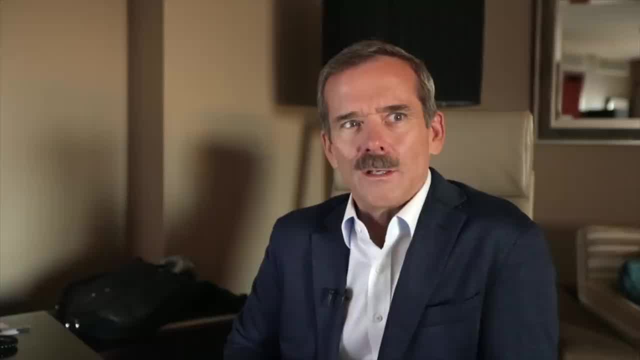 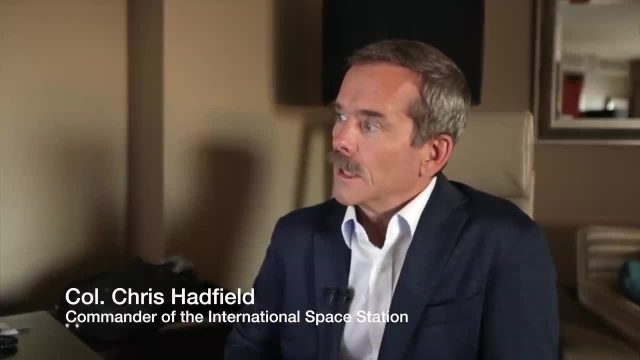 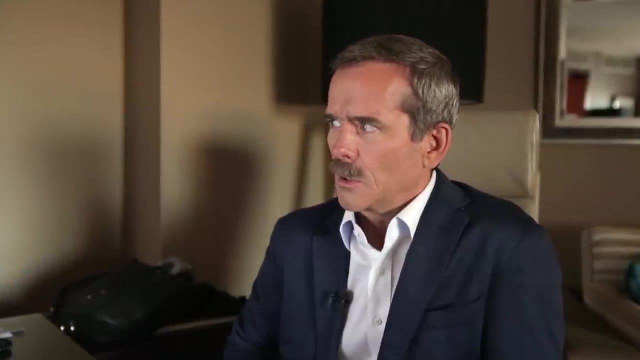 separate bit flips Above the atmosphere. cosmic rays are so energetic sometimes you can even see them Once in a while. you have your eyes closed and you're not asleep yet, and if you wait a little while, you occasionally will see a flash of light and we think it is heavy particles or individual bursts of energy. 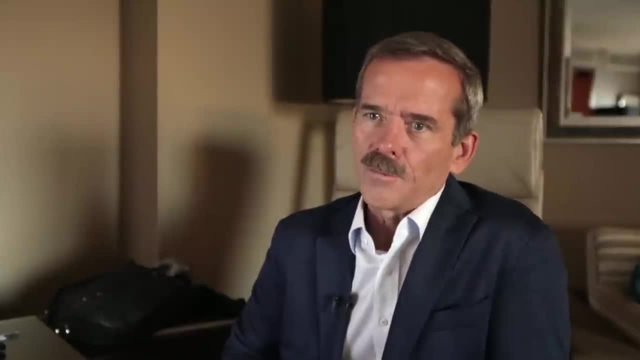 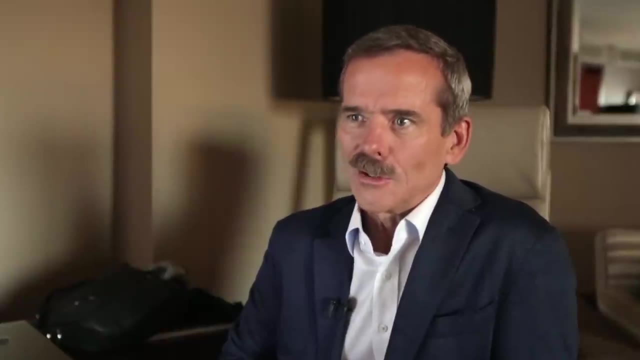 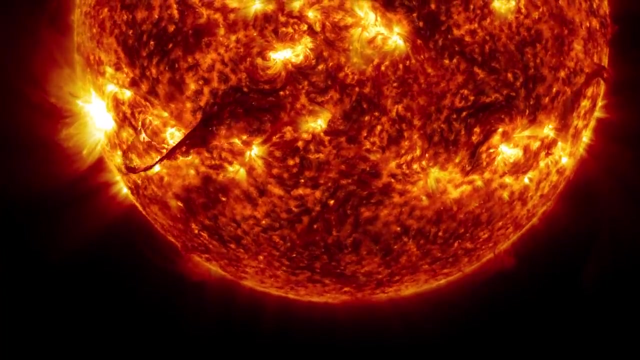 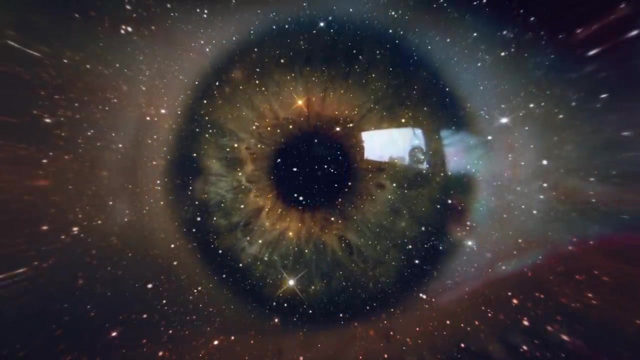 coming from radiation that are either going through the eyeball itself or going through the optic nerve, and the way that your body registers radiation going through it is amazingly enough, by showing you a little flash in one of your eyes just to remind you that You are subject to the radiation of not only our sun, but every star of the universe that is radiating at you. 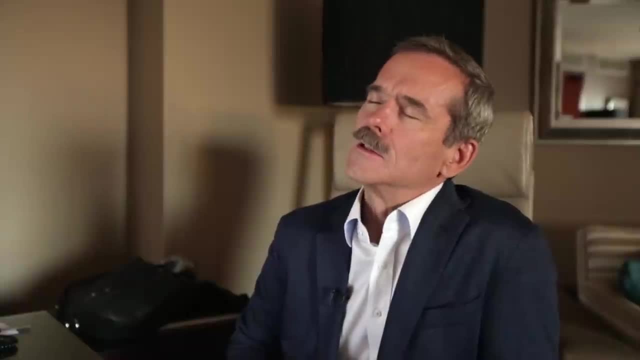 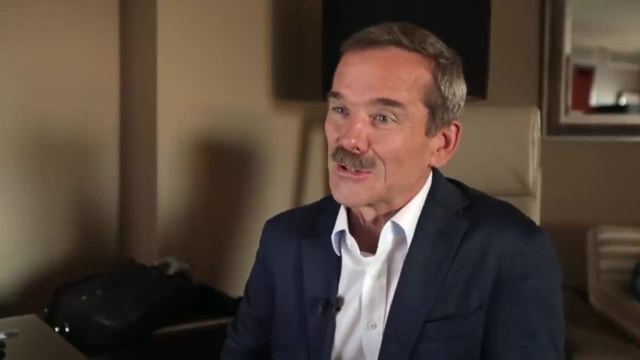 I picture back to the first astronauts who must have closed their eyes and seen that radiation and gone. I'm not going to tell anybody about this because no one's told me about it And I can just imagine the first two guys that said: hey, sometimes I see flashes of light. 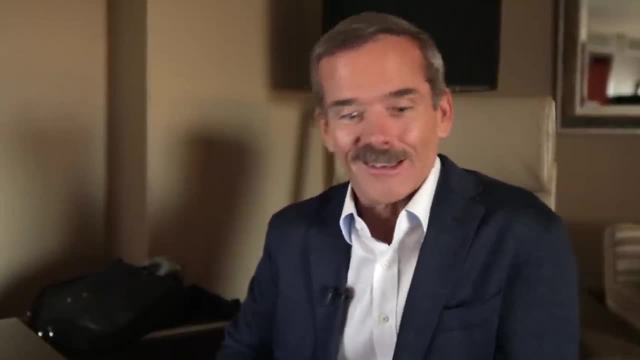 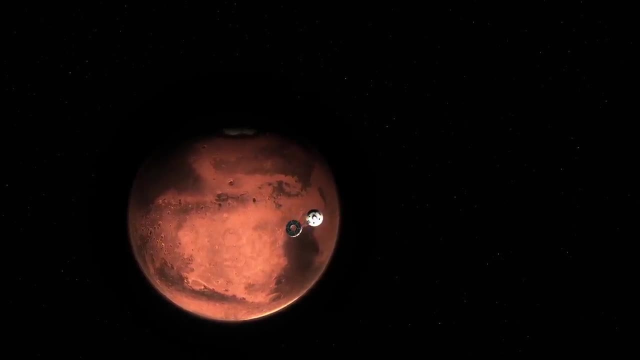 Do you see flashes of light? And then it's: oh, we all see flashes of light. Oh, okay. Well, that's all right then. For missions to other planets, protecting electronics is critical If a single bit of information controls a critical function on your spacecraft, let's say your thrusters. 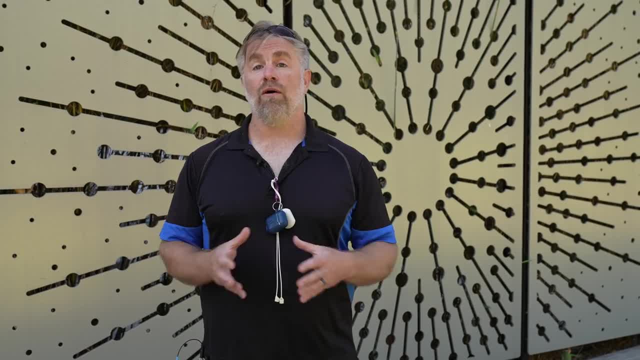 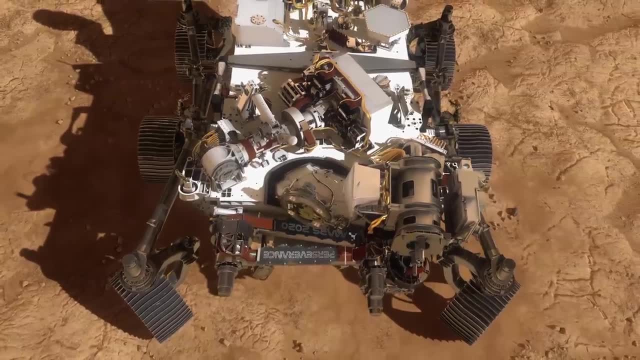 and that goes from a one to a zero, from a on to off or vice versa. you could lose the mission. That's why the computer on the Perseverance rover that just landed on Mars is 20 years old. It's a power PC launched in 2001 with only 256 megabytes. 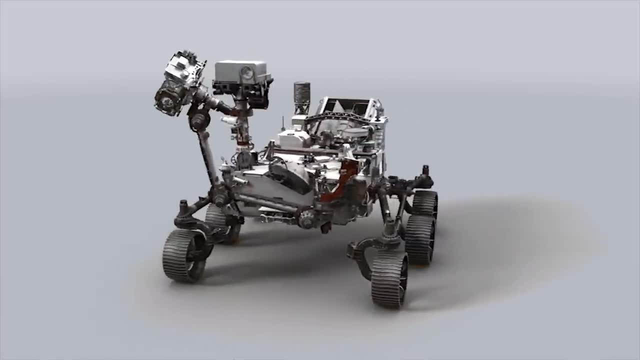 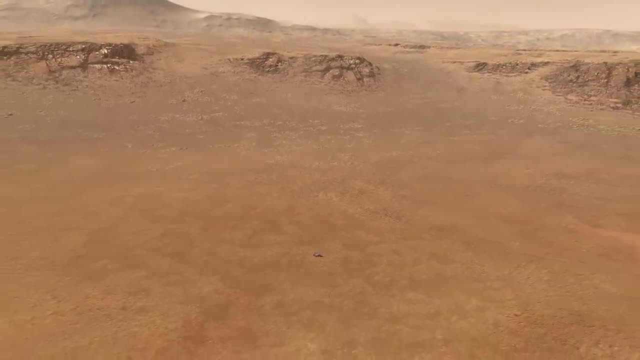 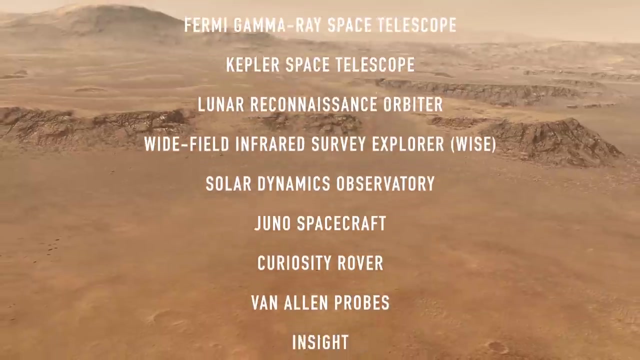 of RAM and 2 gigabytes of flash storage. But it is radiation hardened, meaning the design materials, circuits and software are built to withstand 40 times the radiation of an ordinary computer. It's been used on over a dozen space missions going back to 2005.. 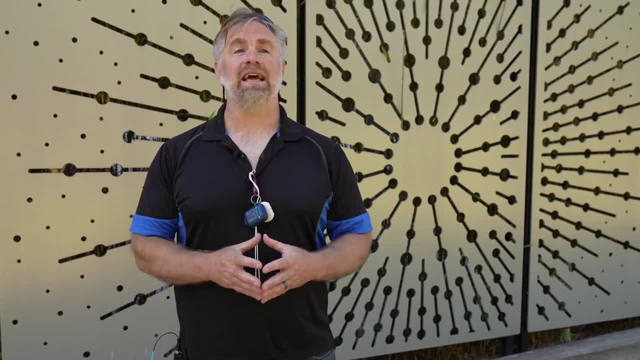 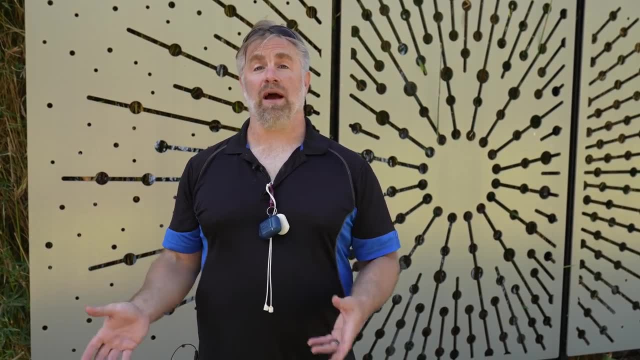 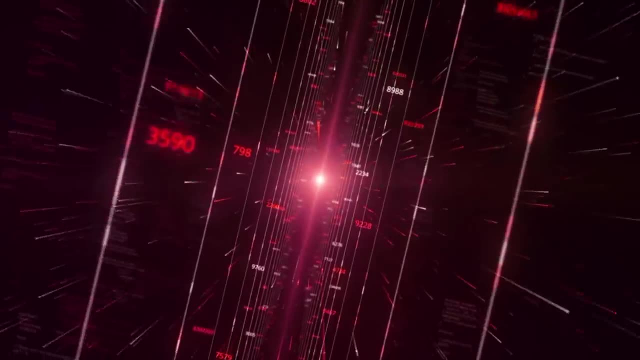 In fact, when we first started doing the power PC testing years ago, the way we did it, we just simply stuck an operating system processor in a beam line where we generate these particles on the planet and look for blue screens of death. You can kind of figure out what's going wrong and try to undo that. 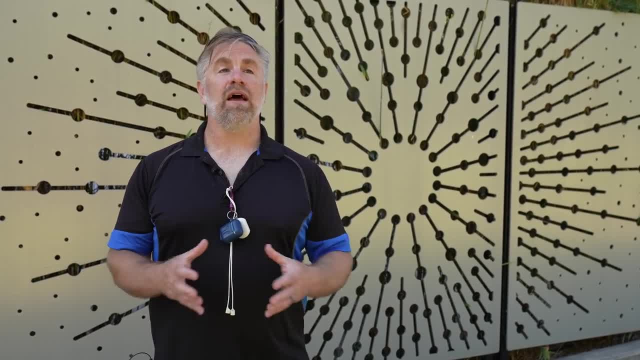 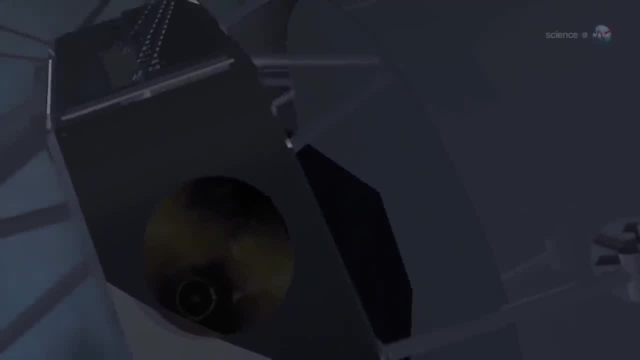 so you don't get to the blue screen of death, because a spacecraft that gets into that mode is basically unrecoverable. As the Voyager 1 spacecraft departed the solar system, one of the ways we could tell was by an increase in the flux of cosmic rays it experienced. 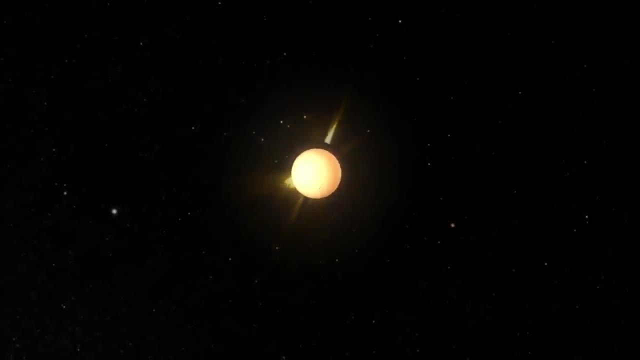 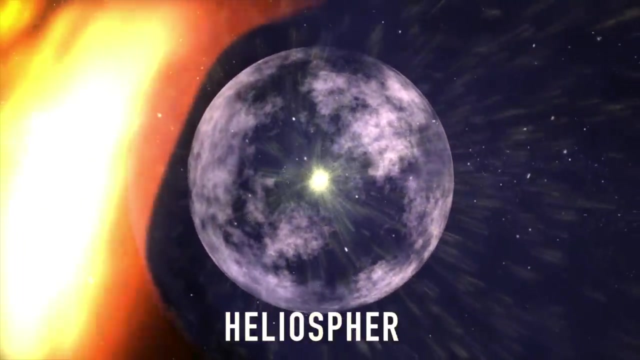 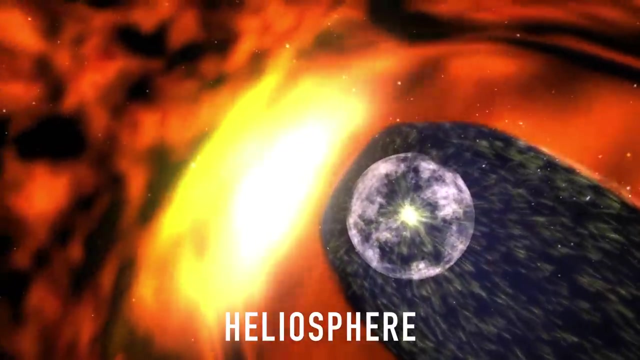 Although on Earth, the particles streaming from the sun and the solar wind are a source of radiation, further out these same particles maintain a protective bubble, the heliosphere. It helps deflect and slow cosmic rays from interstellar space, protecting the solar system from ionizing radiation. 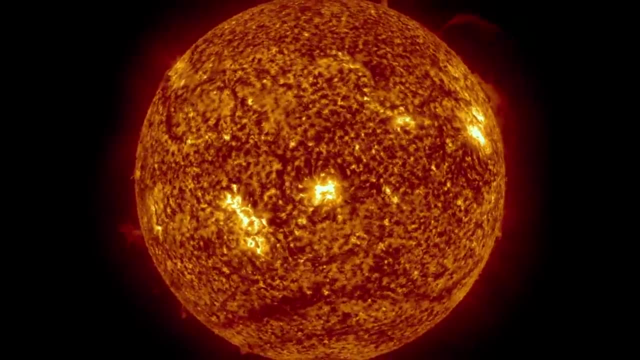 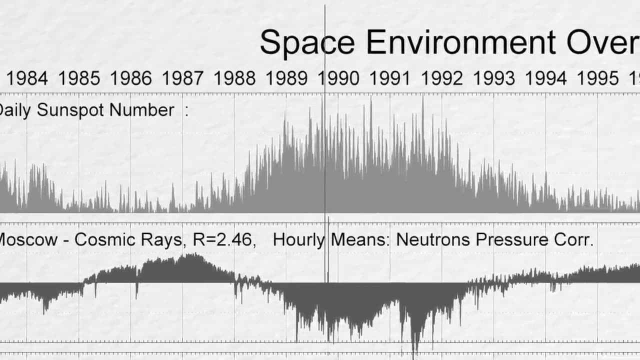 But the Sun has an 11-year activity cycle, so this protection fluctuates. The flux of cosmic rays on Earth is much lower when the Sun is active than when it's dormant. In the history of our planet, cosmic rays may have played a major role in the evolution of the solar system. 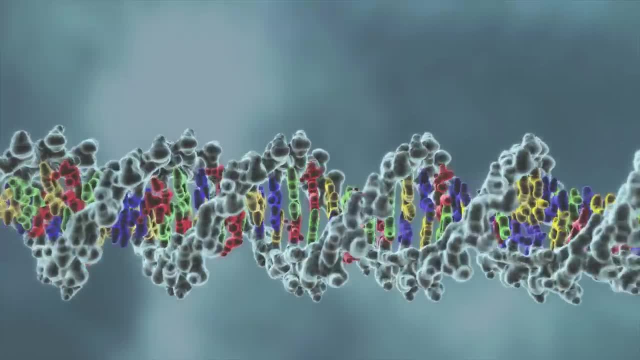 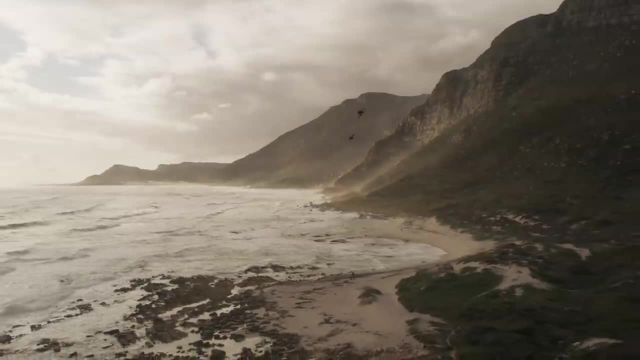 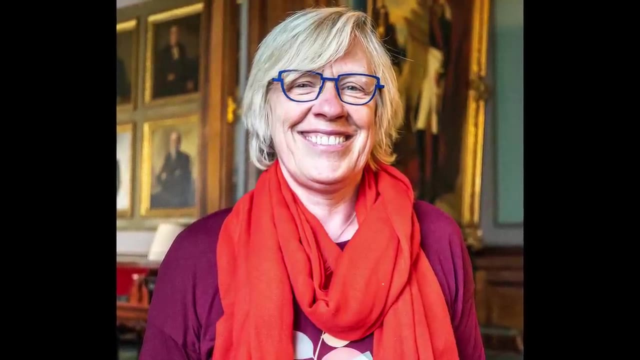 but they have played an even larger role: flipping bits not in electronics, but in the genetic codes of living organisms, providing some of the variation on which natural selection acts. Maria Windevogel is now a member of the Belgian Chamber of Representatives. 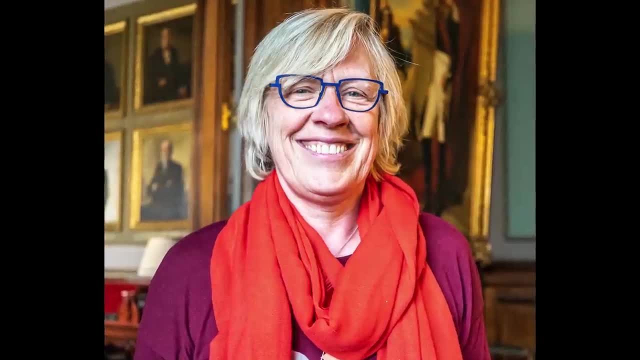 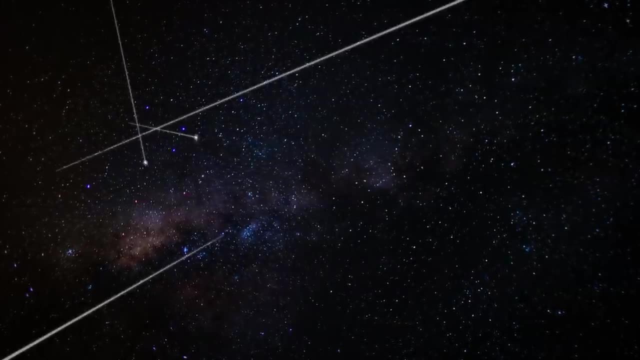 elected by people, not a particle, But her story is a reminder of the zillions of particles winding their way through the universe for millions or billions of years. for billions of years, One of which might at any moment change your life. 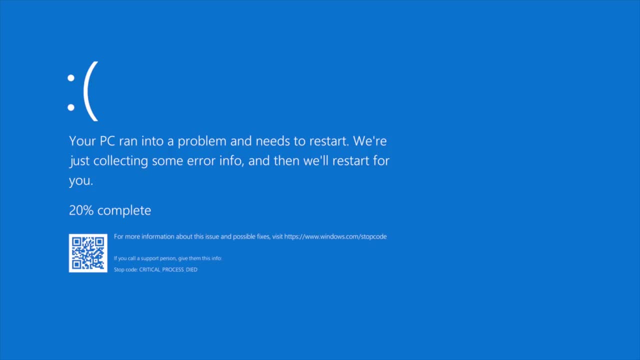 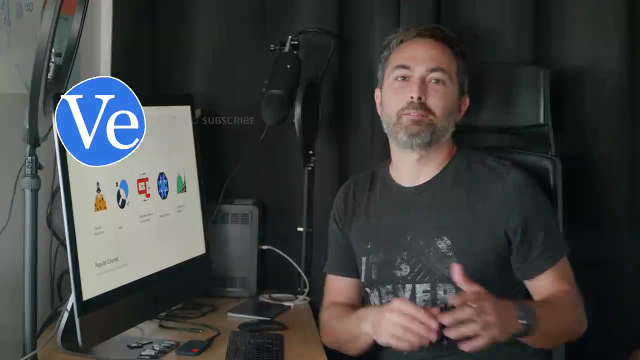 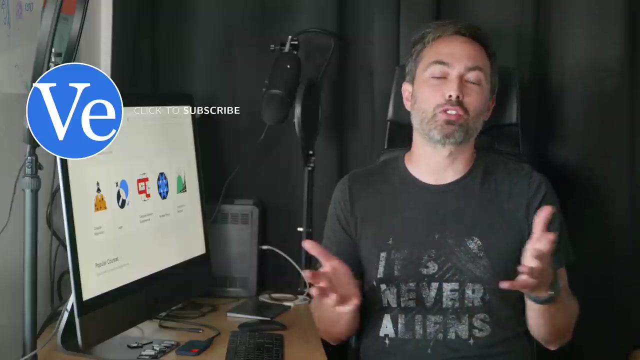 by passing through a tiny transistor and, craaaaaaaaaaaaaaa, Discovering the origin of cosmic rays, or where 4096 extra votes came from, Or how to protect the Mars rover from radiation, requires problem-solving, which is a perishable skill And the best way to keep your volu-. 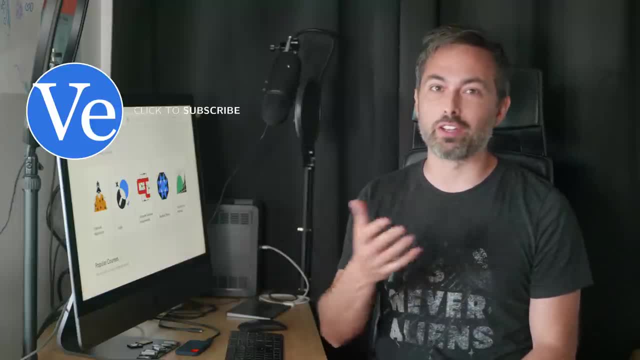 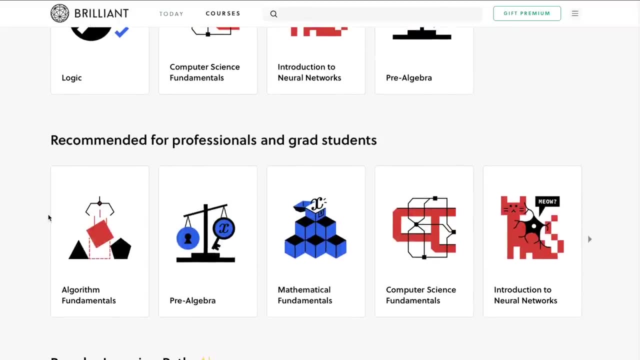 And the best way to keep your volu- to keep your problem solving skills sharp is to solve a diverse range of problems, which you can do with the sponsor of this video, Brilliant. Brilliant is a website and app that teaches you STEM concepts in an interactive way. They have courses on topics from applied computer science. 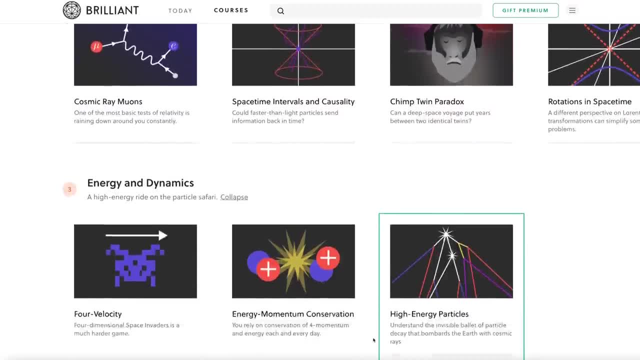 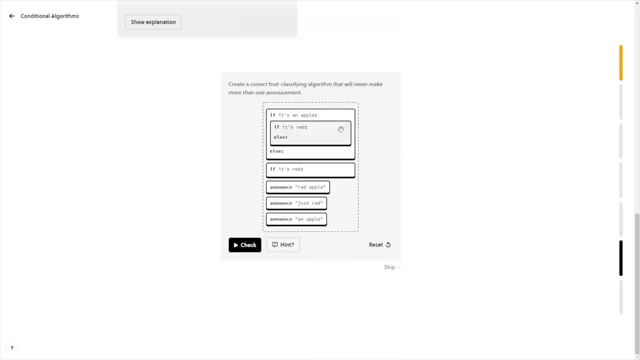 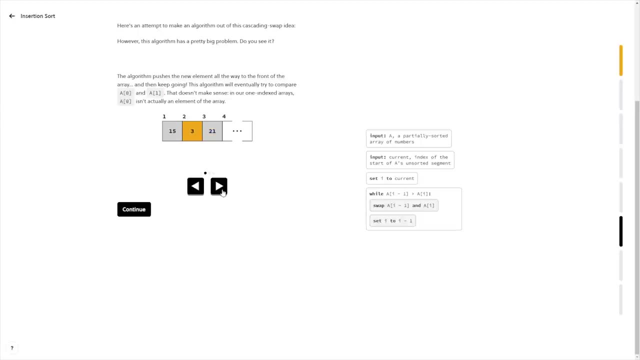 to special relativity. Two courses I would recommend, if you enjoyed this video, are Computer Memory and Algorithm Fundamentals. Brilliant have really upped their interactivity recently, so instead of reading about algorithms, you're taught how to write algorithms yourself. Brilliant engages you in active learning Instead of telling you the right answer, they allow you.